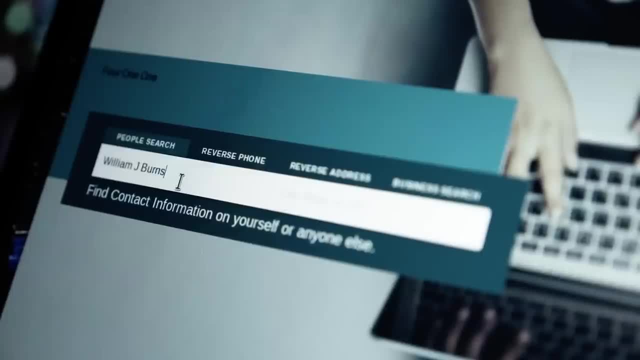 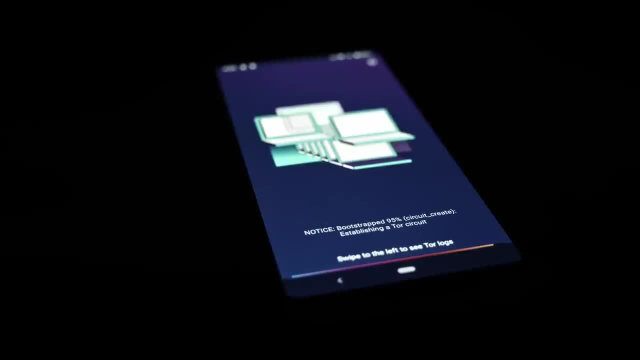 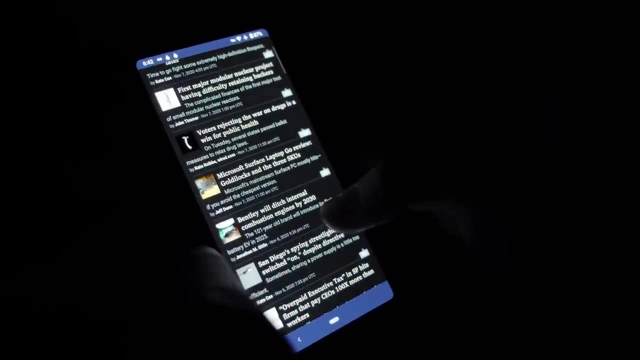 If you're not okay with automated decisions being made about your every move, you should consider getting an anonymous identity. Anonymity is the most powerful mitigation strategy. on a publicly observable network such as the internet, It is the most direct path towards privacy. Anonymity isn't necessarily concerned with keeping your activities confidential. Rather, it is. 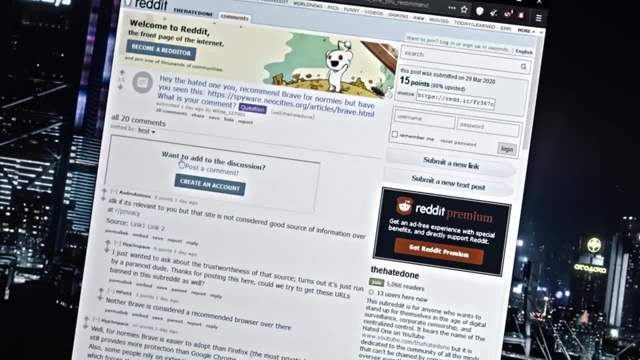 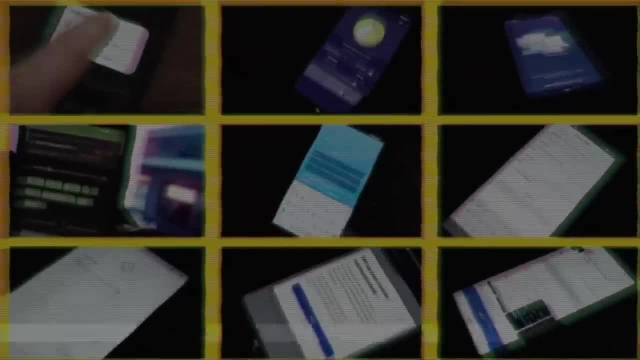 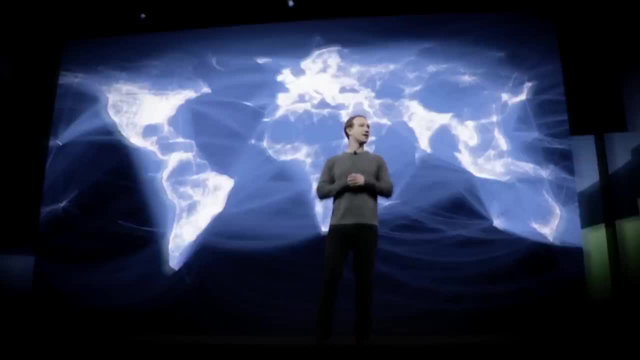 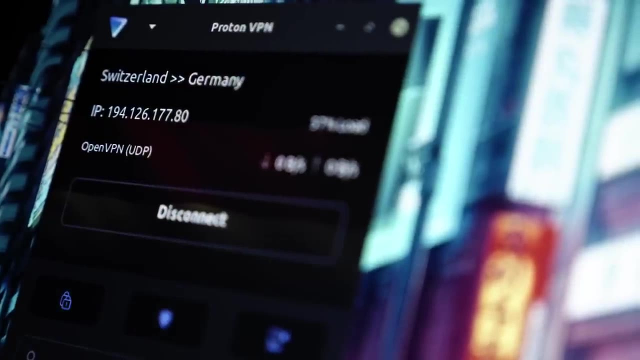 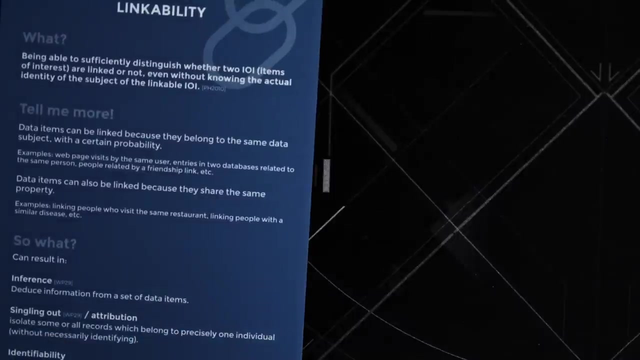 the internet is a privacy nightmare because every action is, by default, identifiable and linkable. that means actions always lead to a unique location and or account on the network, and actions can build a profile over time. linkability and identifiability are your biggest privacy and anonymity threats on the internet. for maximum anonymity, both of these threats 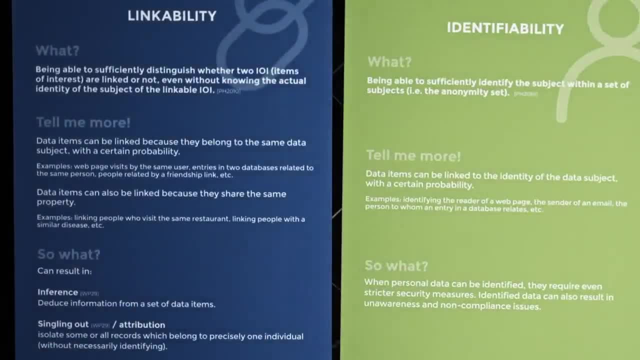 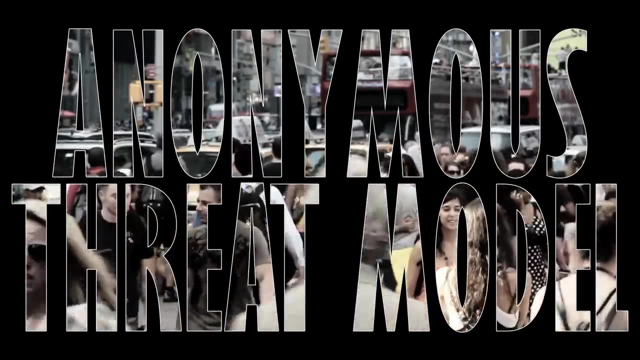 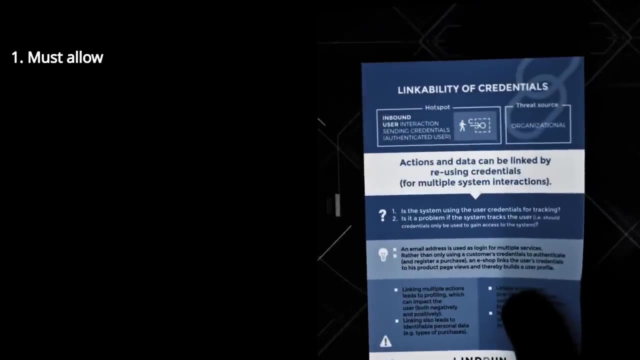 need to be mitigated the fullest extent possible. this means, in order for us to achieve anonymity, every action we take and service we sign up for must meet very specific criteria according to our threat model. in order for a service to be unlinkable, it must allow us to use one-time. 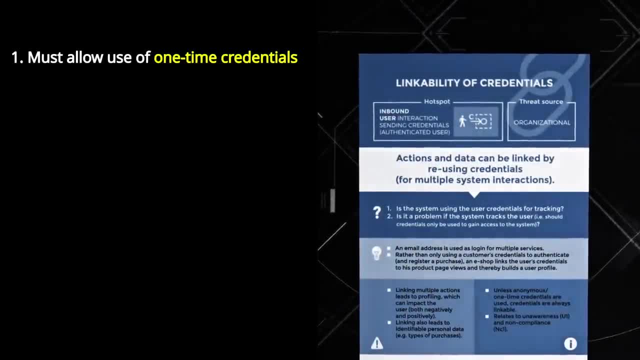 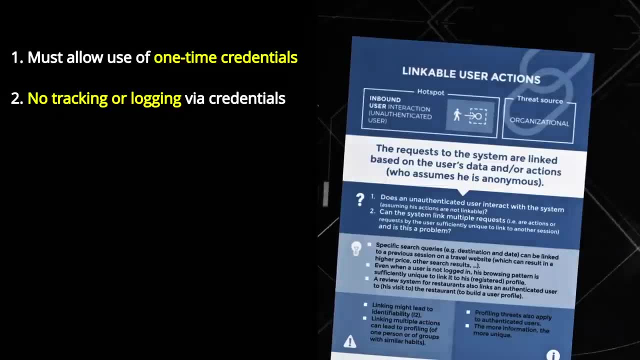 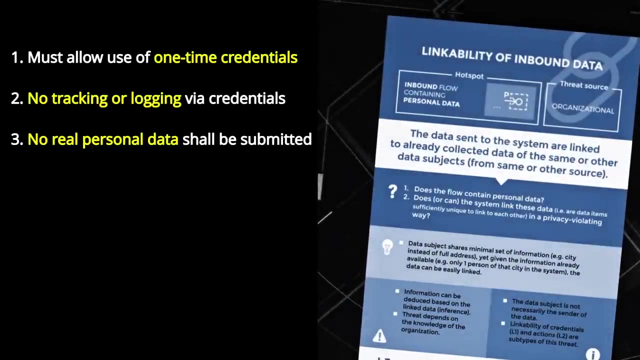 credentials and we must never reuse these credentials. the credentials must not be used by the provider to track or log our behavior, especially tracking of our behavior out of the outside of our anonymous identity. no real personal data should be submitted throughout the entire use of the service. the service must work even on an anonymous overlay network. 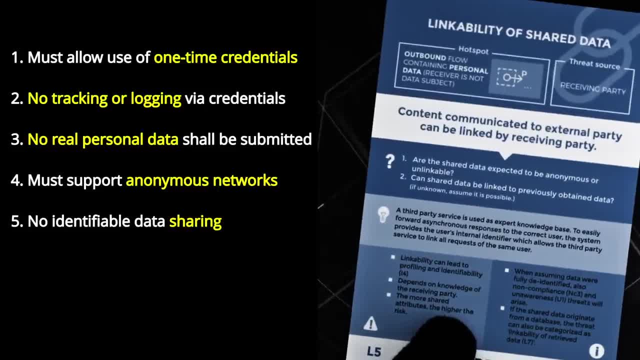 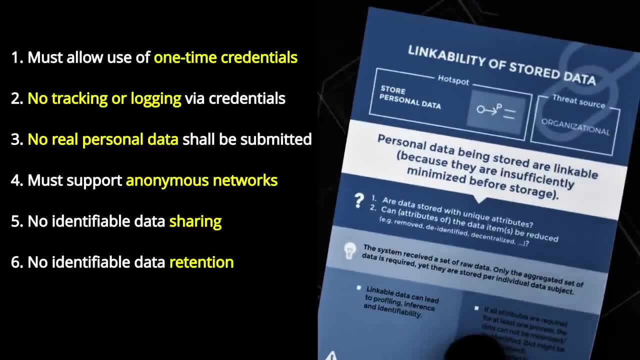 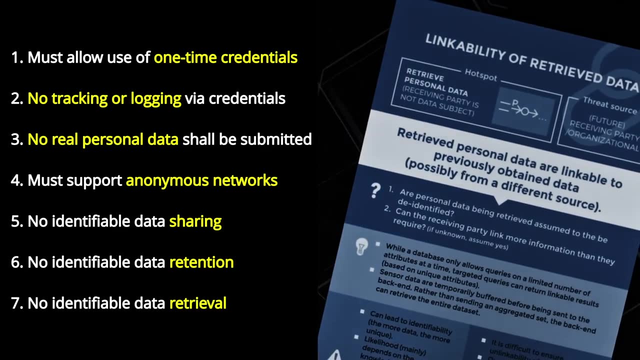 such as Tor. providers of our services shall not share our data with third parties in a way that can lead to our identity. they should retain as minimal data as possible and keep no identifiable logs. it must be impossible for a future party to retrieve, targeting and locating data from public and private network sites and should be required to obtain your 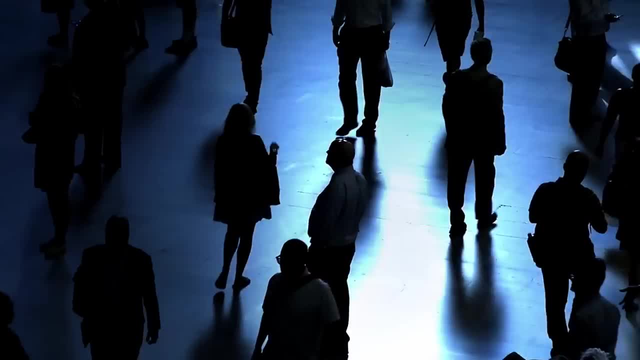 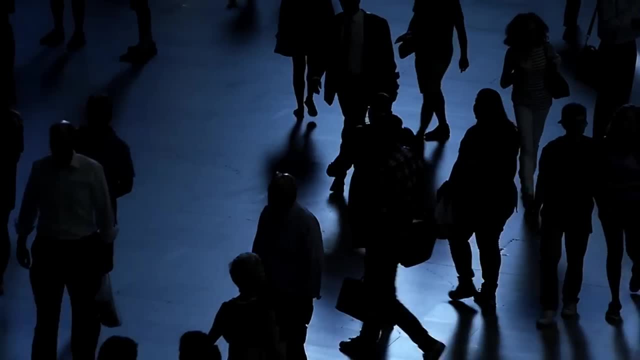 look of are not photos of their identities. outside of our anonymous identity, no real personal data Linkability can lead to identifiability, which can lead to severe privacy violations. To mitigate identifiability on the internet, you have to know and do the following: 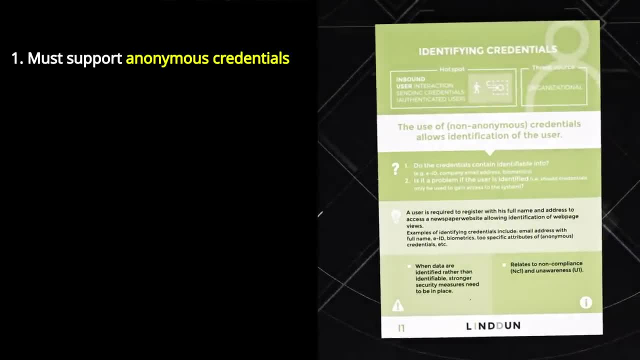 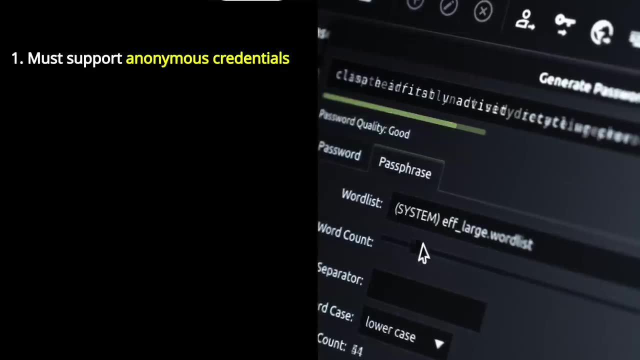 One-time credentials are not enough if they can identify us. The service we use has to support anonymous credentials: Pseudonyms, nicknames, aliases, random strings that have nothing to do with our real name or location. The service should not have any prior knowledge about us. 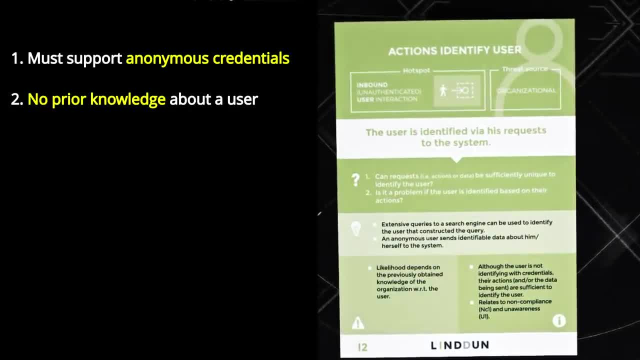 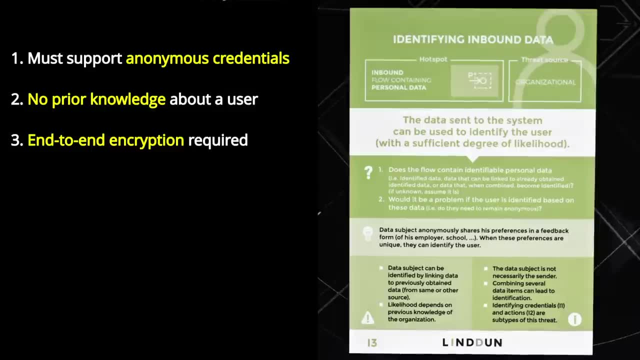 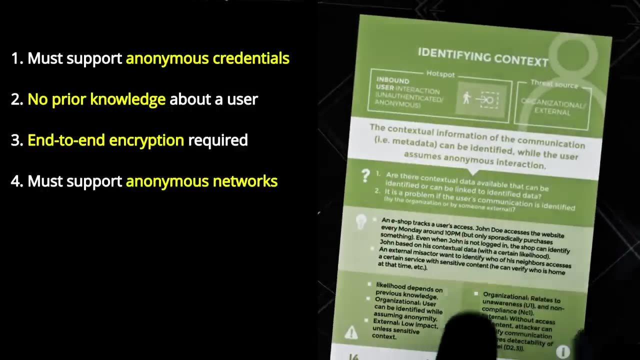 If it does, we need to be extremely cautious and compartmentalize our identities. Account creation and use of the service must not require personal information and all content has to be encrypted with a key. only the user can access. The service must be fully functional over an anonymous overlay. 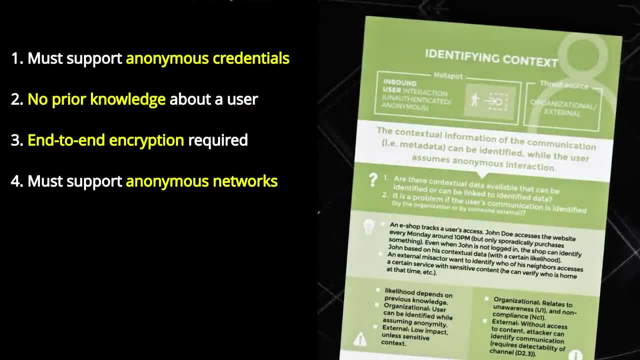 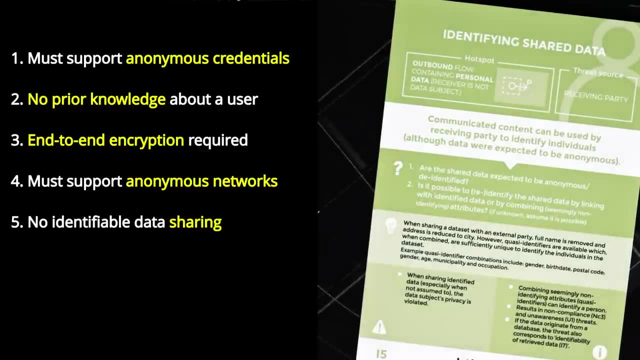 network or, by the very least, a reputable VPN. The provider must not share our data with third parties, nor acquire additional data from external sources that can help them link our projects to the internet. The service must be fully functional over an anonymous overlay network. or, by the very least, a reputable VPN. The provider must not share our data with third parties, nor acquire additional data from external sources that can help them link our projects to the internet. The service must be fully functional over an anonymous overlay network or, by the very least. 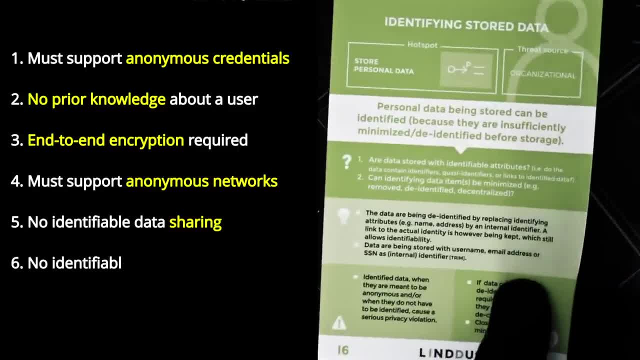 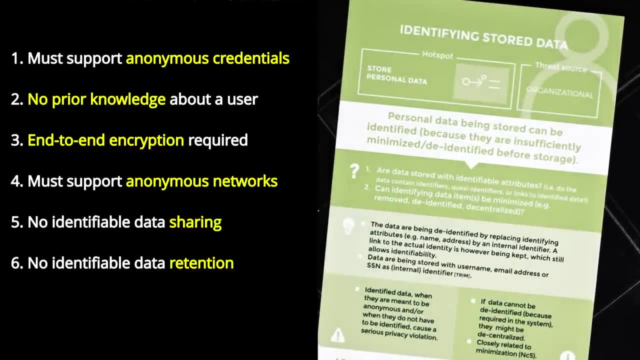 a reputable VPN. The provider must not share our data with third parties, nor acquire additional data from external sources that can help them link our projects to the internet. The service should retain as minimal data as possible, keep no identifiable logs, and any retained data must be sufficiently. 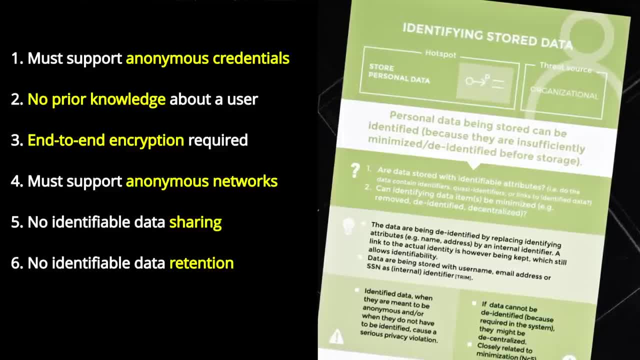 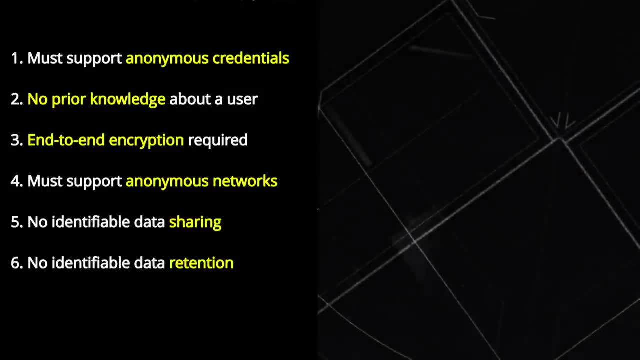 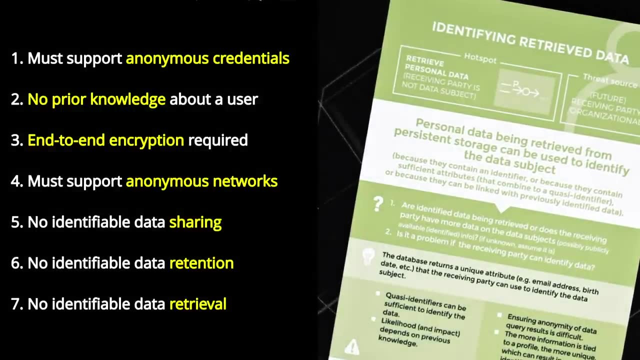 de-identified. This is a very hard assumption to make, so we should give these services as little functional information about us as legally permissible And, lastly, it must be impossible for a future party to retrieve identified data, which means we have to carefully read privacy. policies of our services. The service must be fully functional over an anonymous overlay network or, by the very least, a reputable VPN. The service must be fully functional over an anonymous overlay network, which means we have to carefully read privacy policies of our services. The service must be fully. functional over an anonymous overlay network, which means we have to carefully read privacy policies of our services. The service must be fully functional over an anonymous overlay network, which means we have to carefully read privacy policies of our services To know how much of the 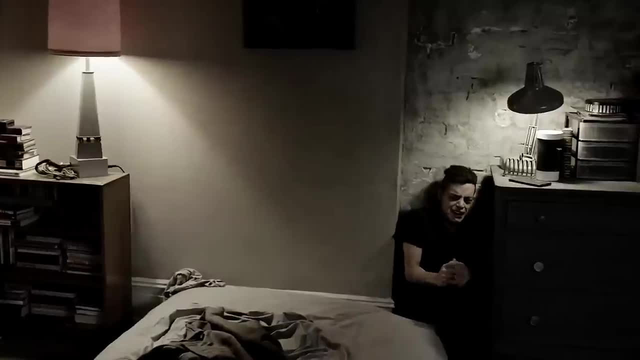 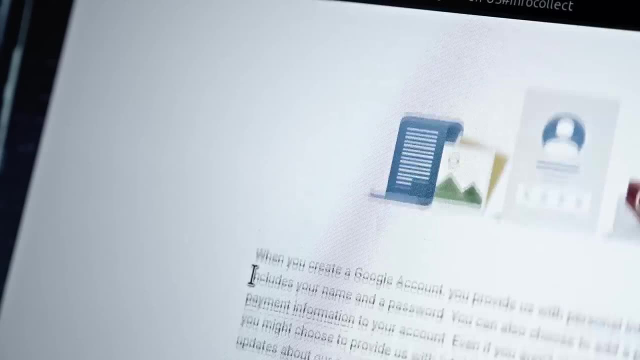 harvested data could lead to our identity. Don't worry, I'm here with no life and friends, and I'd love nothing more than spending a portion of my life reading privacy policies. to bring you this tutorial for free, Speaking of which I'm going to lay out some very specific services. I 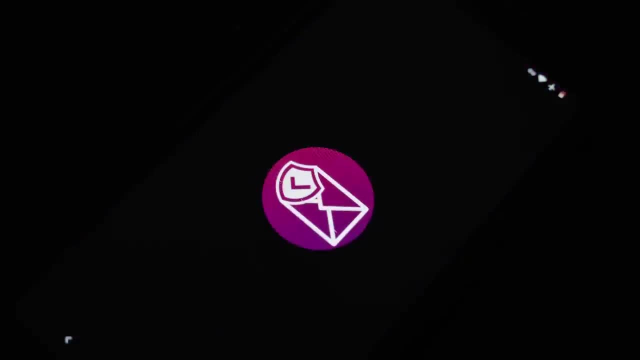 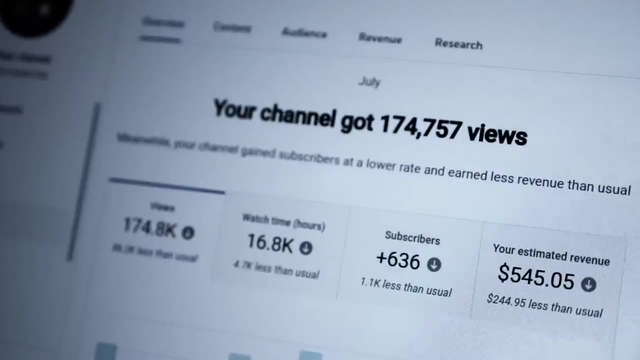 recommend for this setup. I'm not affiliated with or sponsored by any of these, so there is no financial interest that could taint my advice. YouTube, on the other hand, has rewarded my efforts with the lowest ad revenue yet and a community guideline strike as a bonus. 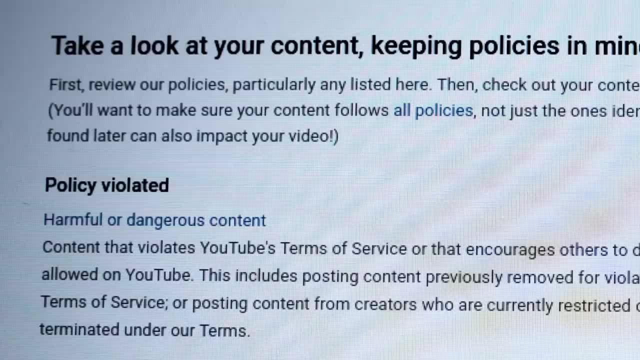 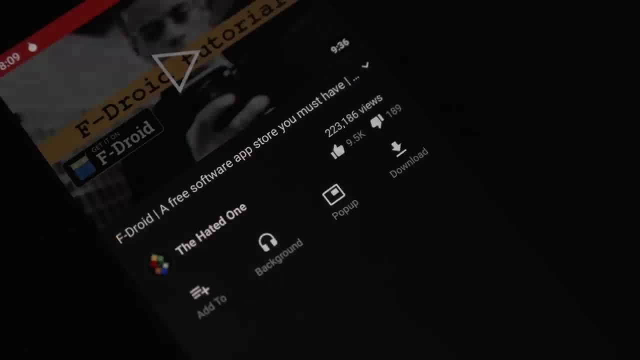 They deemed my new Pipe tutorial out of all things dangerous and harmful, with no reason as to why. It was a video that taught people how they can watch YouTube videos with Google Ads and trackers completely for free. Now that video was deleted by YouTube, Think. 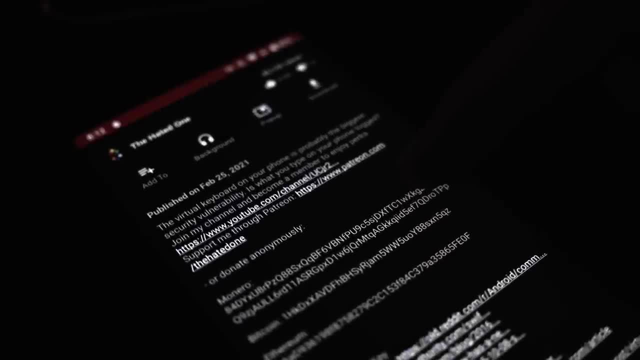 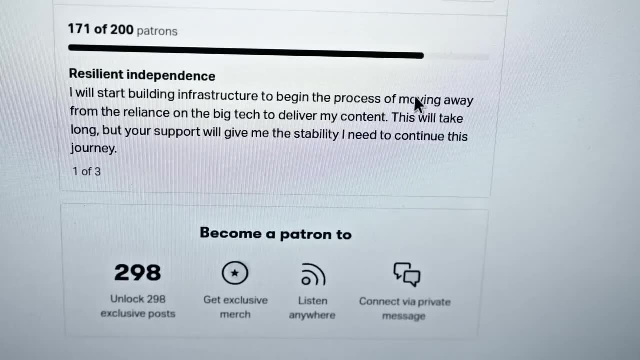 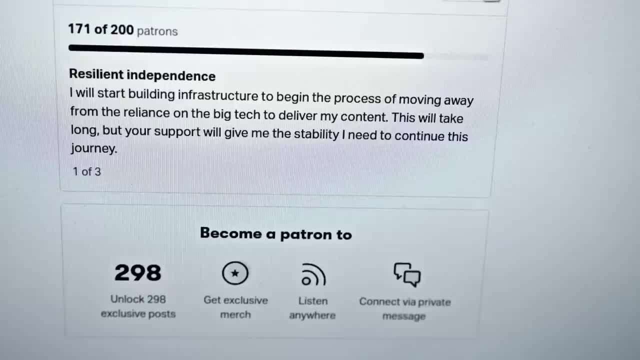 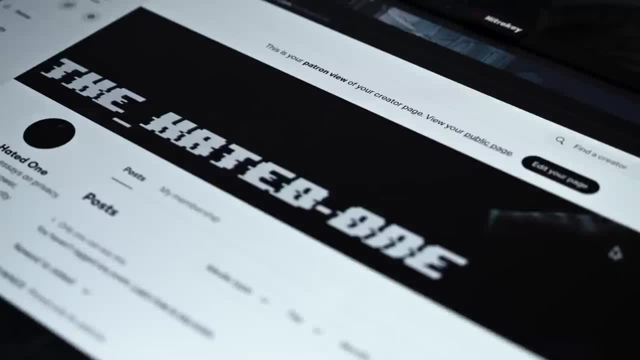 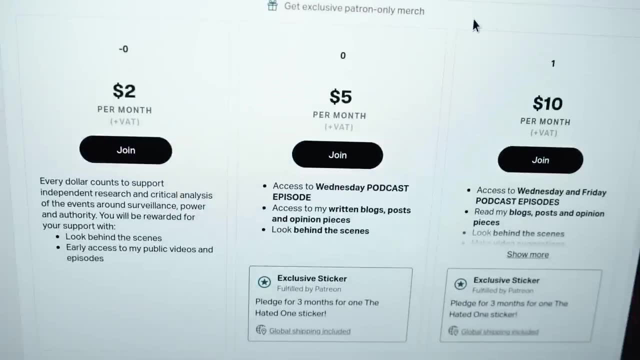 slash TheHatedOne. I know these self-promotion plugs are annoying, so if you do sign up for my Patreon page, you'll be rewarded with over 100 Patreon-only podcast episodes and will get text versions of all of my new videos and tutorials. Thank you. 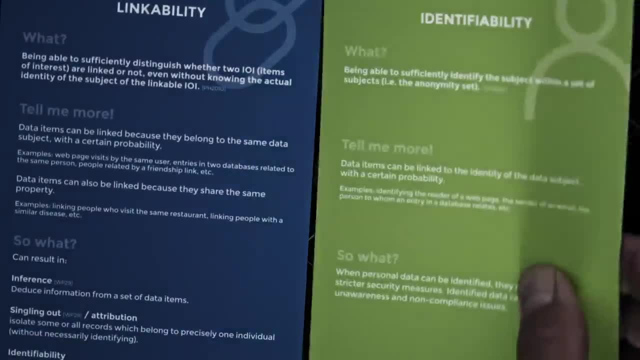 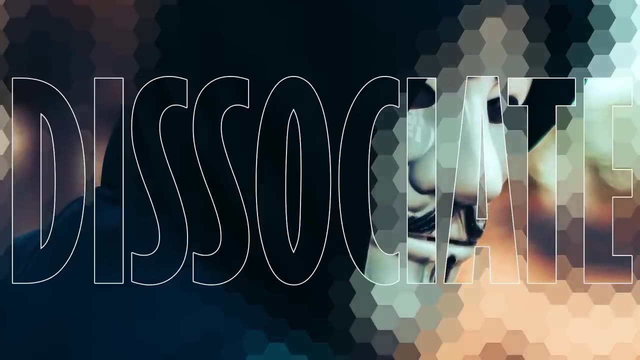 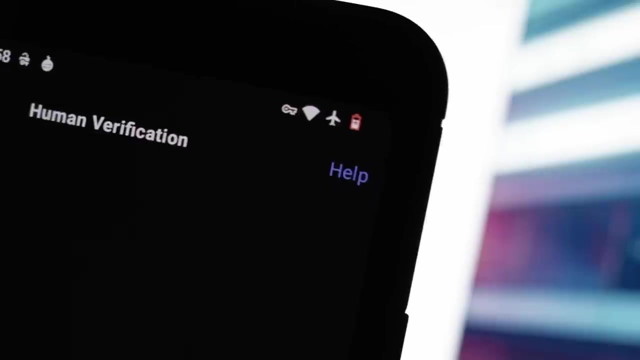 So now let's mitigate all of the linkability and identifiability threats to our anonymous identity. Our first step with any service will be to dissociate our account details from our personal information. The most common account identifiers are phone numbers and email addresses. We need to count them into threat hotspots, even if they are used just to. 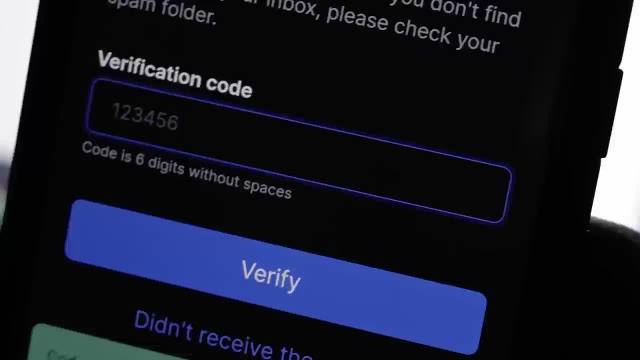 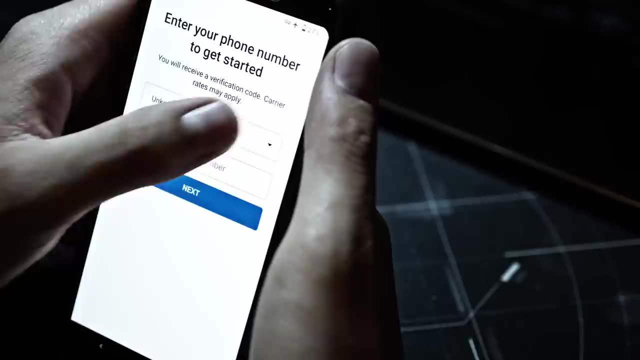 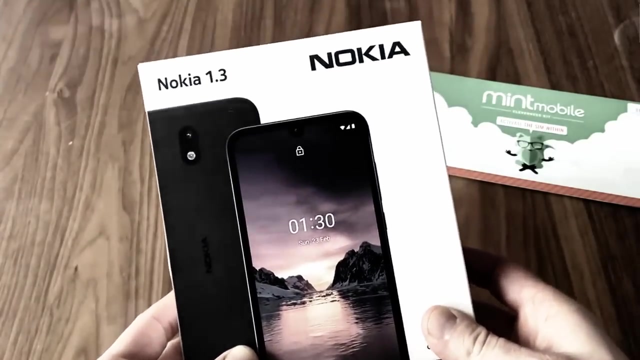 confirm human verification. to prevent spam accounts, I would advise against using any service that requires a phone number, because it is going to be very difficult to create and burn new anonymous identities on as-needed basis. Phone numbers can be obtained anonymously, but you have to be in the right jurisdiction to do so. 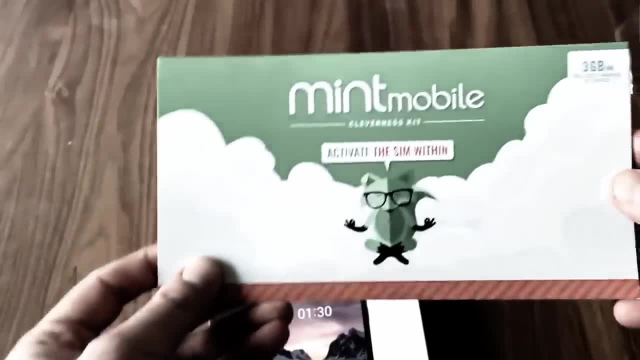 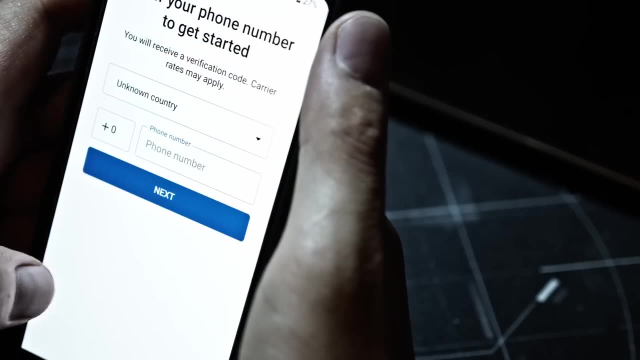 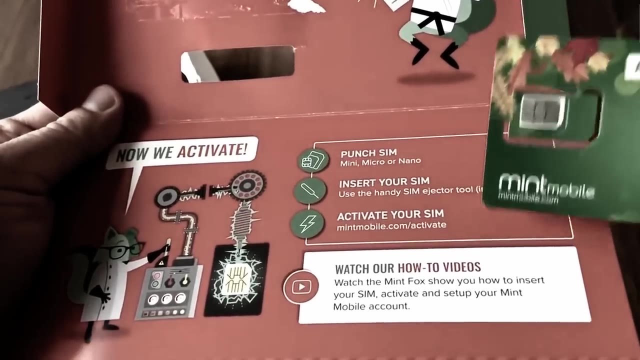 If you live in a country where you can't get a prepaid SIM card without submitting a government ID, you should avoid a service that requires a phone number. We will talk about those in a bit. If you can't obtain a SIM card without an ID registration, you need to purchase not only a 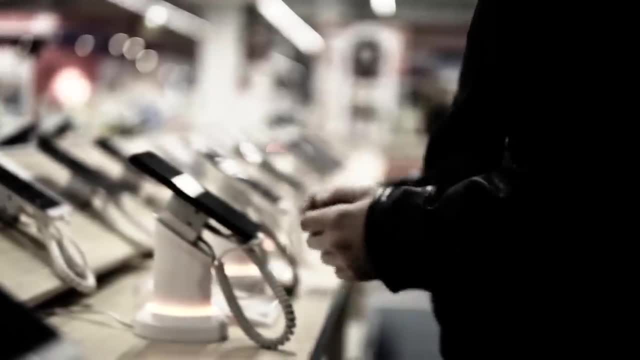 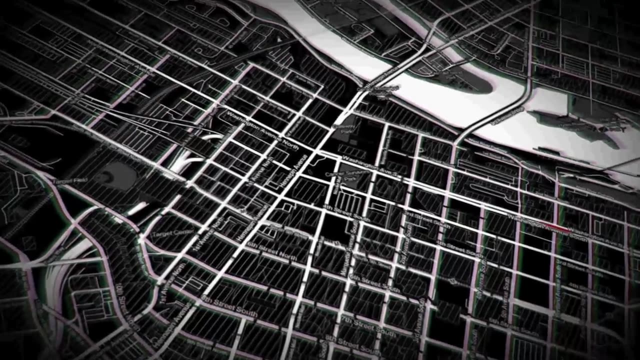 new SIM card, but also a new phone device. The purchase, activation and all use of this anonymous phone is only allowed to happen far enough away from your home or work address If you're in a country where you can't get a prepaid SIM card without submitting a government ID. 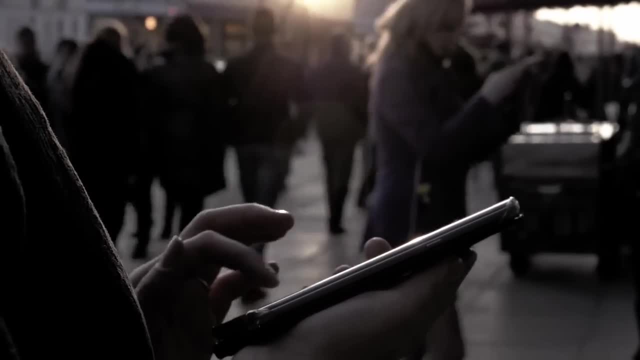 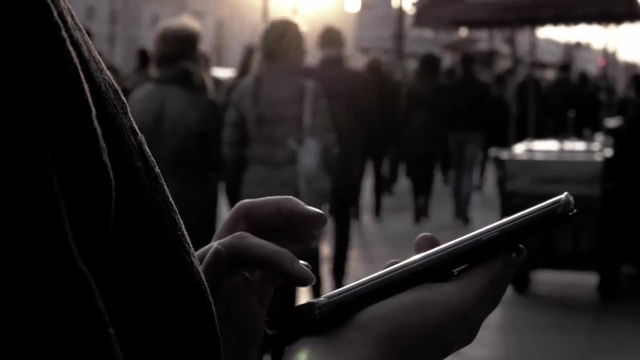 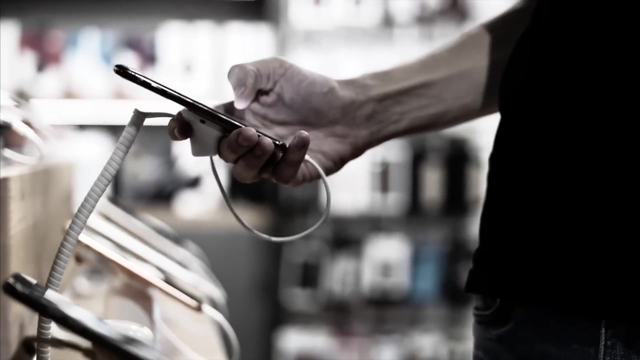 Your phone's carrier will immediately recognize your phone's unique IMEI and it will associate the new SIM card with your personal identity and location. This is why you need both a new SIM card and a new device. Any cheap one will work, as long as you pay in cash in a physical store. I have an in-depth tutorial on how to be anonymous. 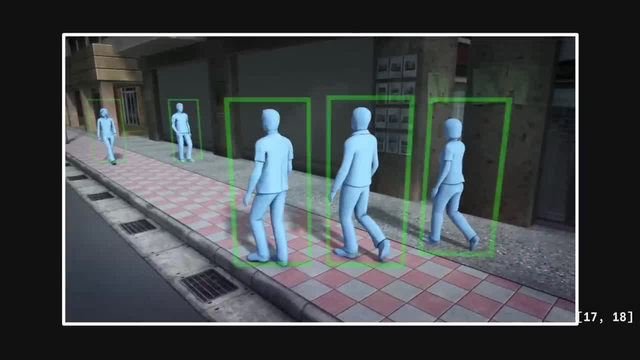 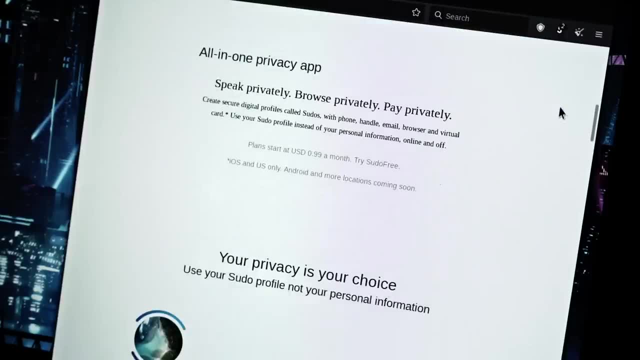 in the streets. that is extremely relevant to this scenario. if you need to obtain an anonymous phone numberорт, Don't trust your mobile phone number when you need to select a phone number If you are not voice over IP services, as these aren't anonymous nor private. They're mostly. 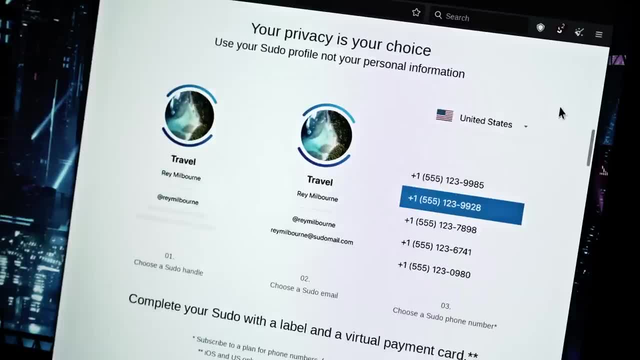 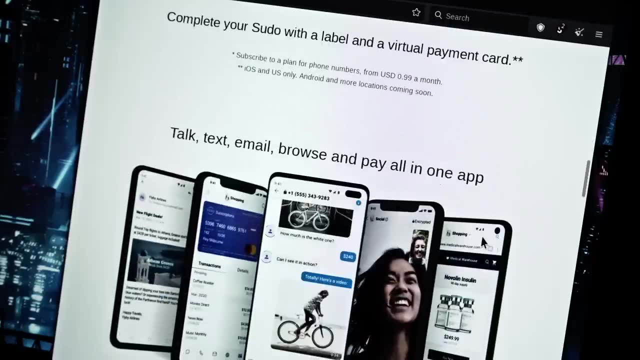 good at preventing spam abuse, but the voice over IP providers don't allow anonymous accounts with numbers that actually work For pretty much any service that we're gonna recommend here. voice over IP numbers won't work for account verification. An anonymous email address, on the other hand, will serve us. 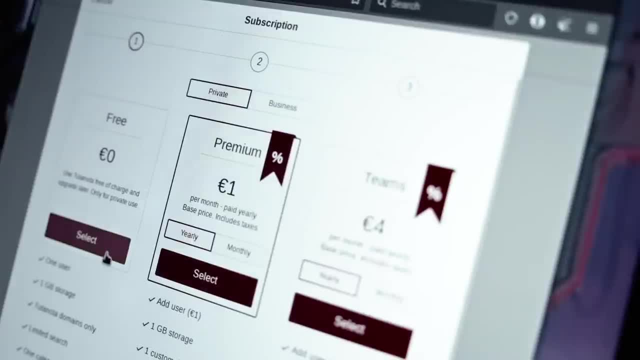 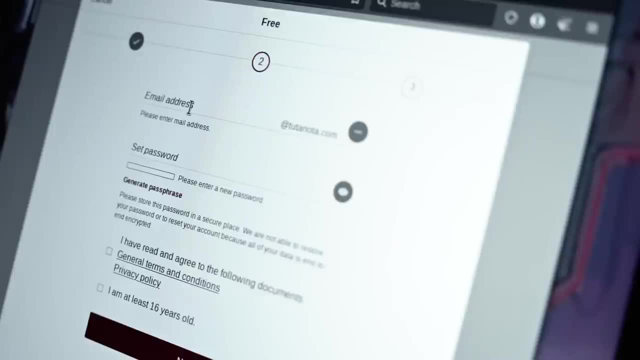 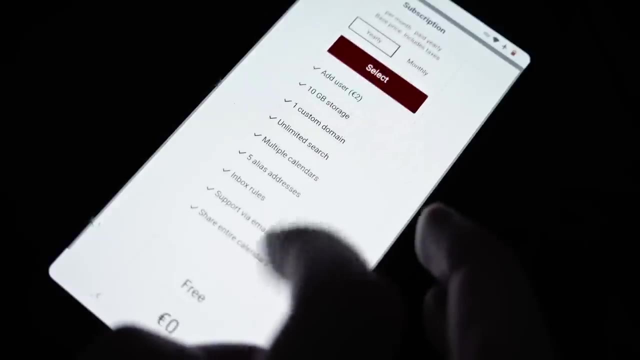 extremely well for multiple use cases. For our benchmark, we want a provider that allows us to create a service with no identifiable credentials, no personal data, and permits account creation over the anonymous Tor network. This is necessary to prevent our ISP from knowing the websites of our service. 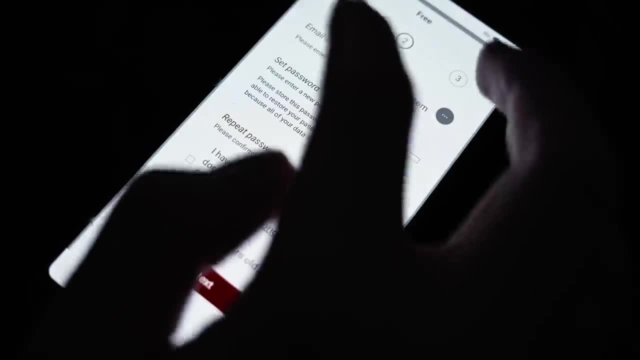 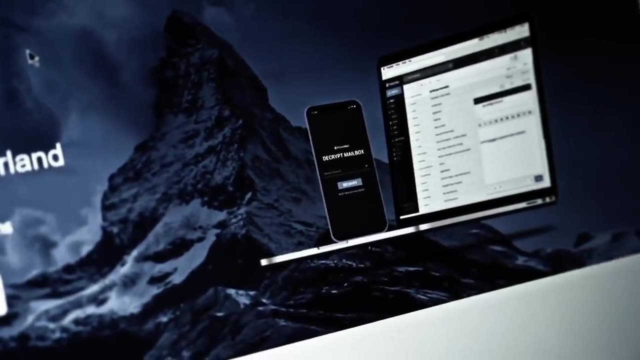 providers and to prevent the websites from knowing our true location. The most often recommended free private email is protonmail, Unfortunately, too many times with an affiliate link. This is a problem because if you attempt to create a protonmail account over Tor, you'll be slapped with the. 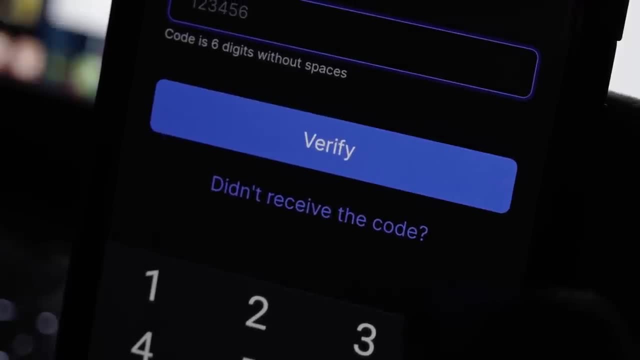 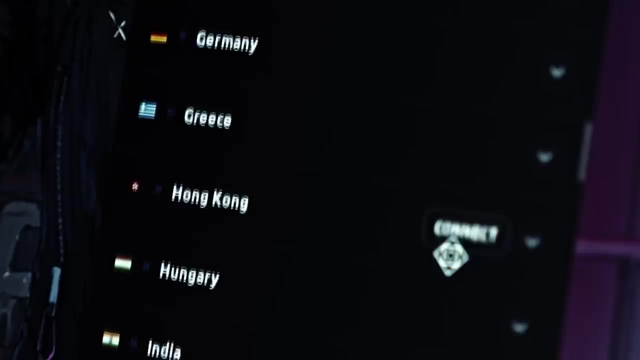 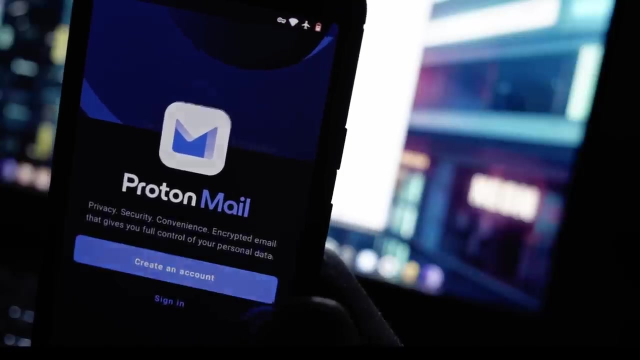 requests for human verification by SMS or an external email address. in a lucky scenario, A third-party catch request or an external email will likely be required, even if you use a VPN. For this reason, I actually don't recommend that you start with a ProtonMail account for anonymity. We should start with another. 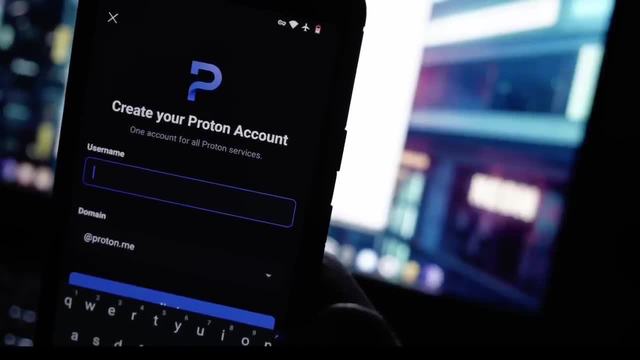 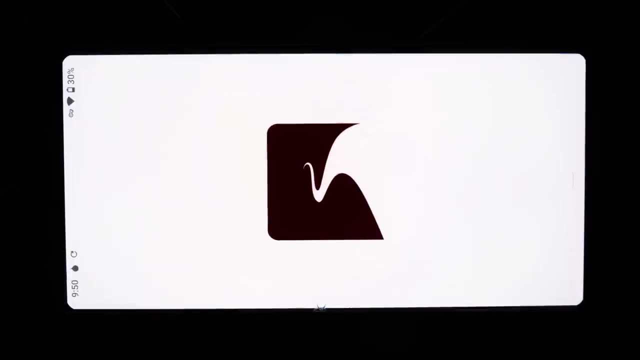 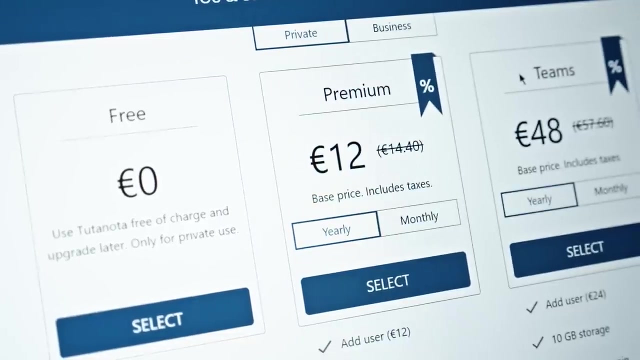 free email provider that is much more suitable for our intentions and use it to sign up for other accounts, even ProtonMail. This other private email is Tutanota, based in Germany. This much less known email provider is also encrypted, but permits account creation over Tor. The only caveat is that you might get your account suspended for 48 hours if you exit from a node that got flagged for abuse. However, in most cases you should just be able to wait it out and your account should be fully functional then. I have tested this many times and I always got my account automatically approved. If you create an 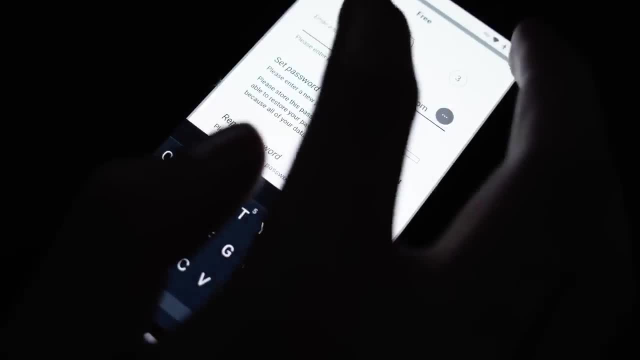 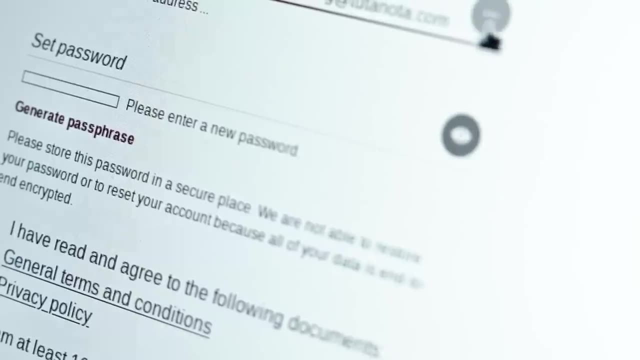 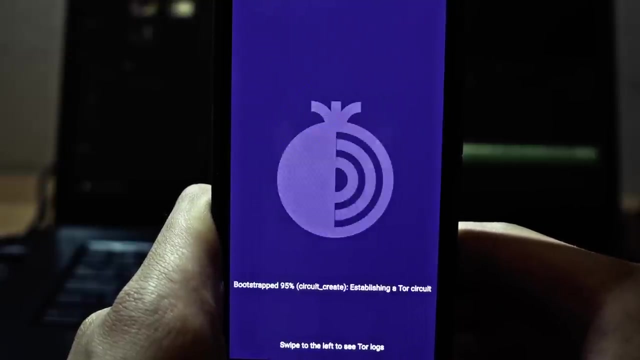 account over a reputable VPN. it is very rare to get the 48-hour suspension. You can create your anonymous account in one of two ways. Both of these matter depending on your setup. If you want to create an anonymous account on your personal device, I recommend doing. 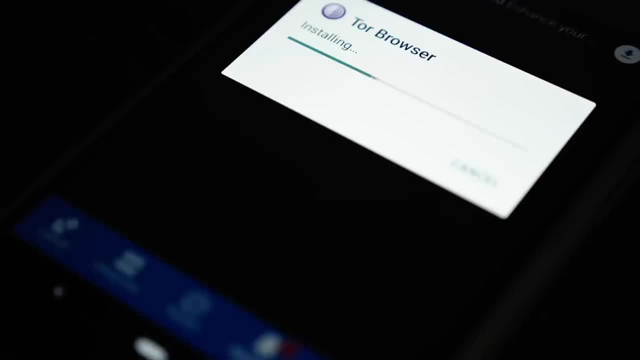 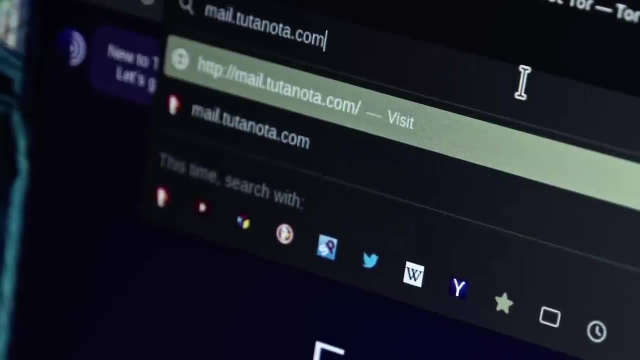 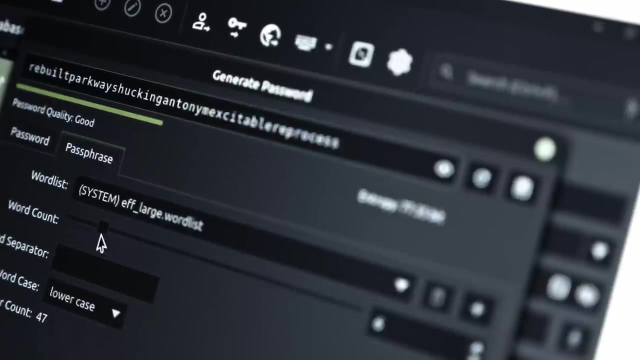 it through the Tor browser. First download Tor into your phone or laptop from the official App Store or torprojectorg. Then go to mailtutanotacom and follow the instructions to create an account. To make unidentifiable and unlinkable credentials, I recommend creating a. 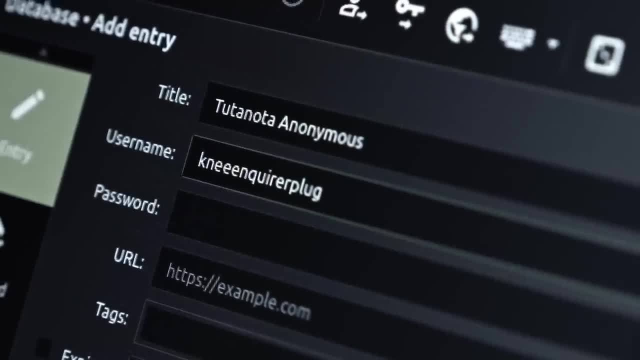 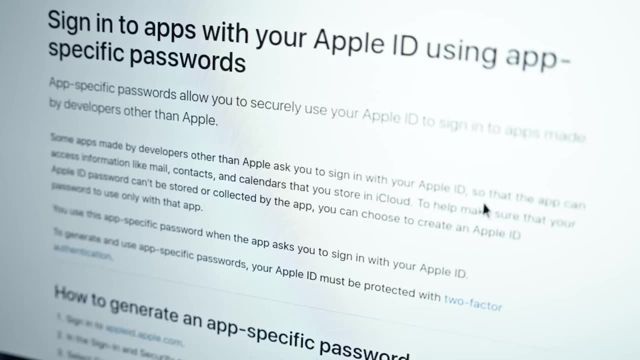 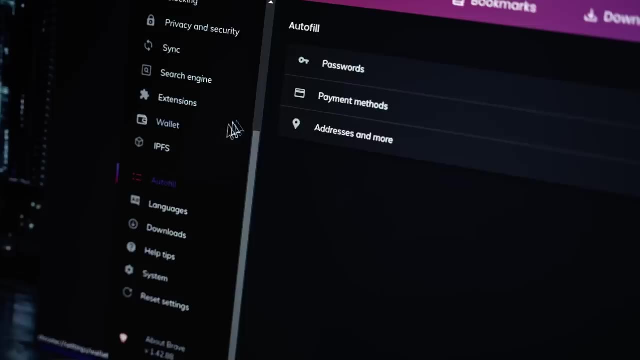 unique username-password combination with a password manager. I use keypass xc because it doesn't need an account to create a database. It is not advised to use a proprietary password manager, especially those that come with your platform, such as Apple or Google, or your web browser, because you don't want these. 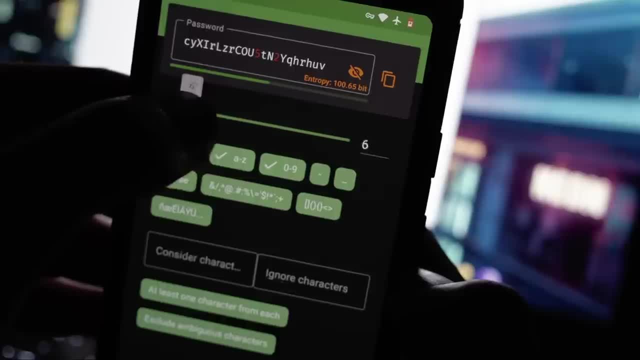 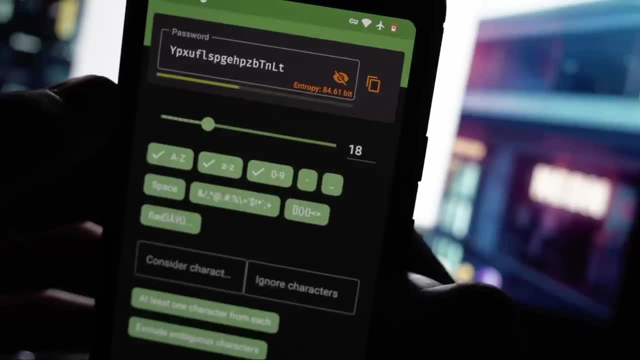 platforms to track what websites you create accounts for. Use your private password manager to generate a unique string for the username as a password, as well as for the password, to create credentials that are truly random and unlinkable to you. When you finish the setup, your account will either be: 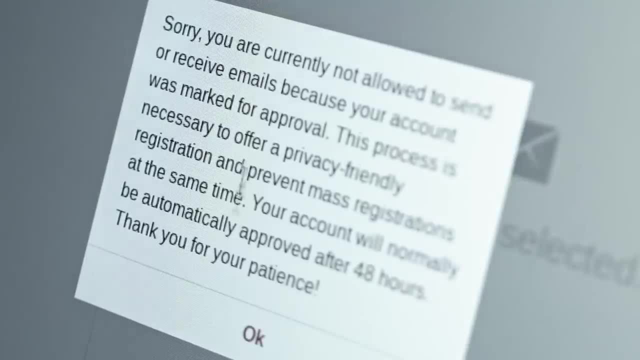 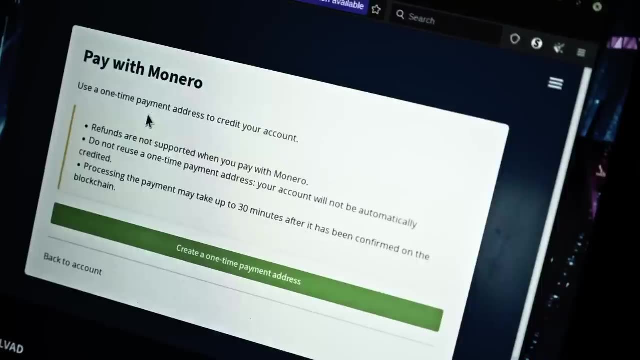 opened immediately, or you will be slapped with the 48-hour suspension. If you don't wait that long, I recommend creating an account over a VPN that you purchased anonymously. The only two I'd recommend are Mulvat or iVPN. You can speed up the. 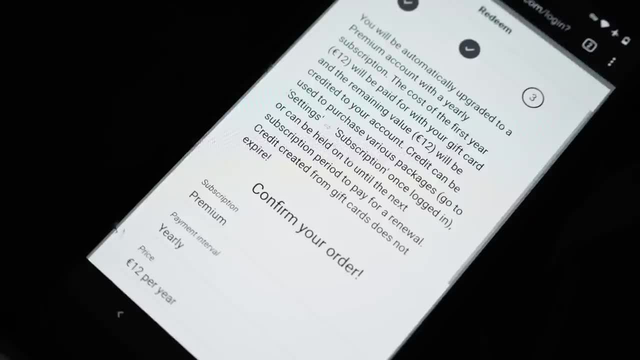 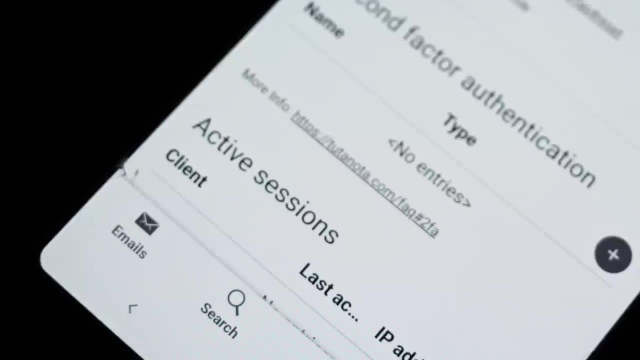 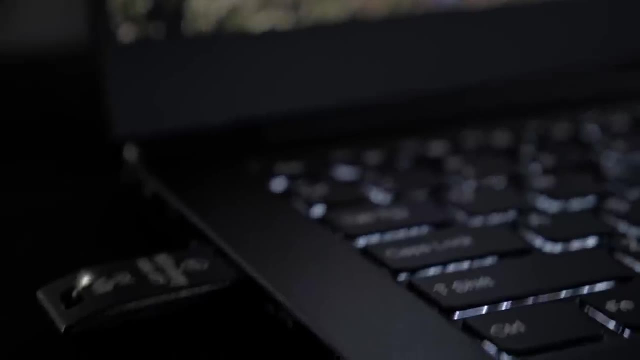 registration process. if you opt for a paid account and use Bitcoin or Monero to obtain an anonymous gift card for Tutanota Now, with your account created, before you do anything else, set up second-factor authentication. Go to settings and add a new 2FA method If you have a FIDO authentication key, 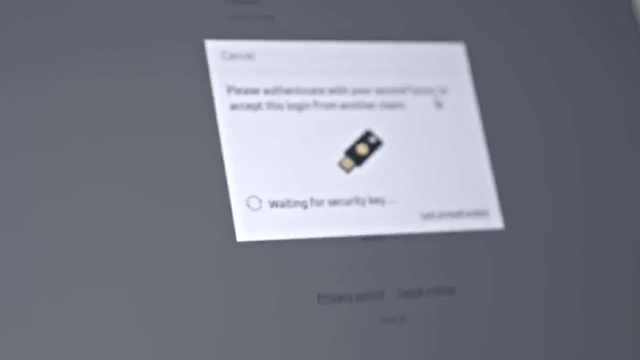 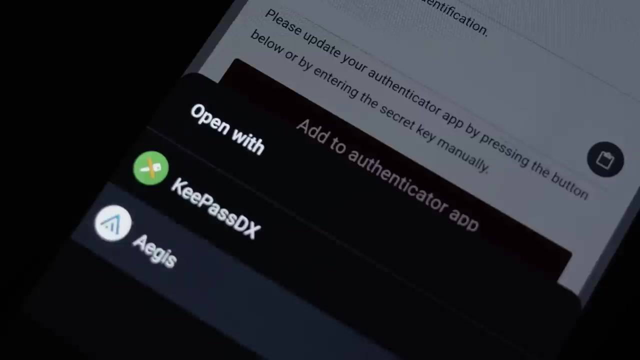 this is a superior method. Alternatively, you can use an authenticator app such as Aegis to generate one-time passcodes for your second factor. I'm going to mention 2FA here only, but remember to enable second-factor authentication for all of your current or 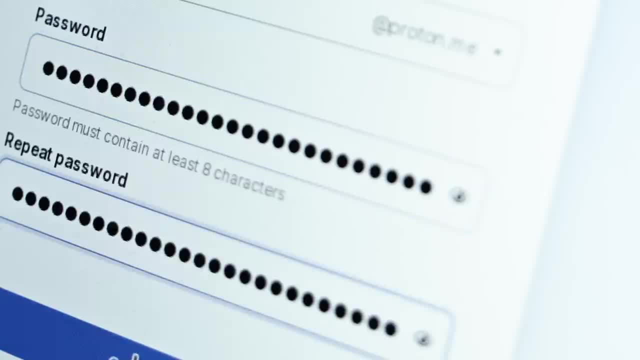 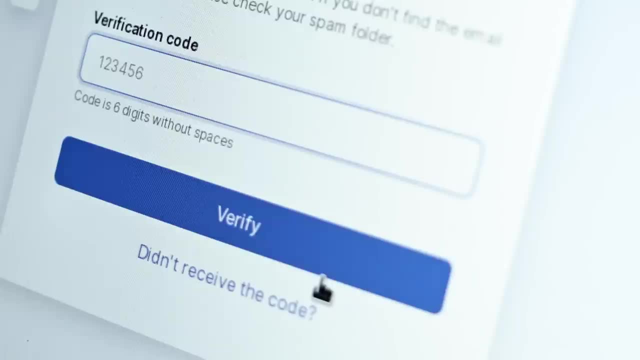 future accounts. Now we can use our Tutanota account to sign up for other services anonymously. If you want to get an anonymous ProtonMail account, just follow the steps for account creation and use your anonymous Tutanota email address for human verification. 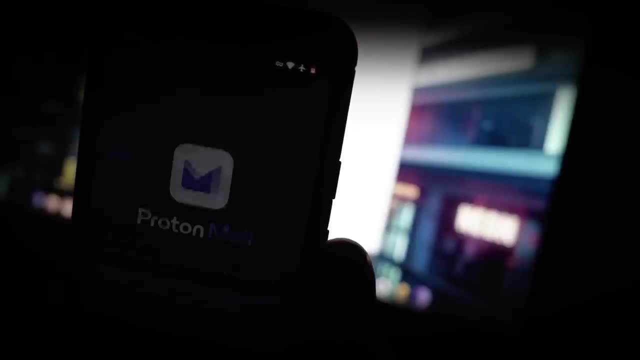 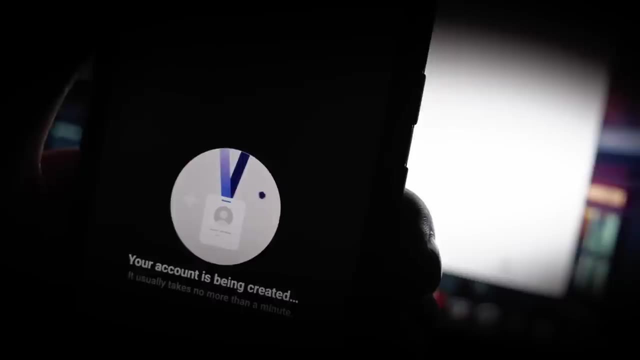 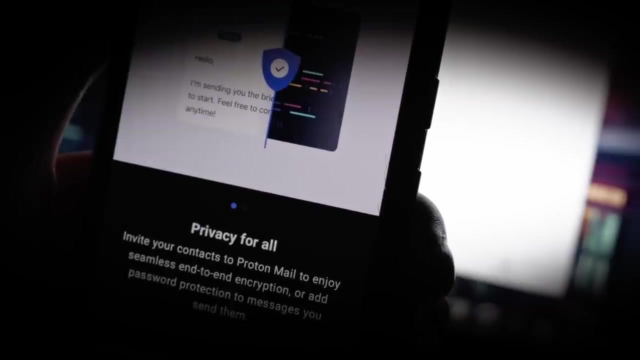 There is a more secure way of creating these email accounts, but this is where you really need to walk the extra mile to protect your anonymous identities. If you use a native mobile app on an up-to-date phone, you will be in a much more secure environment than a browser on a laptop. 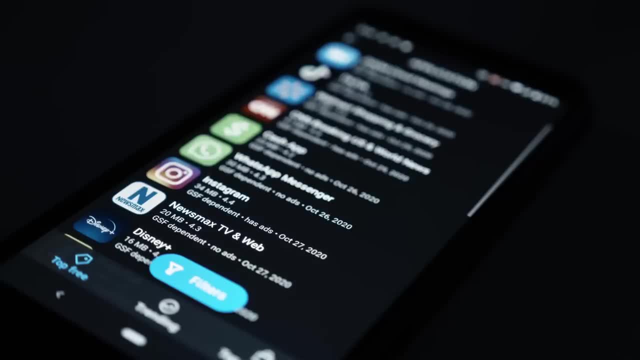 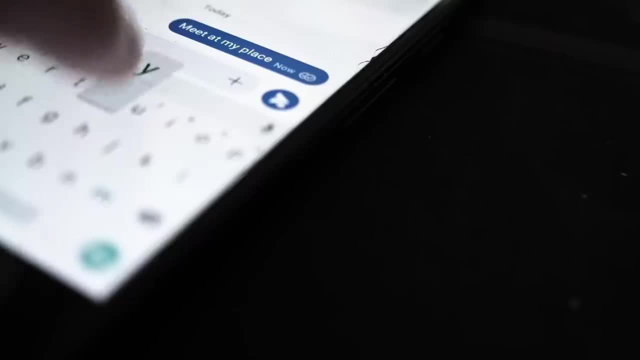 There isn't enough space to discuss all the details why that's the case, but what's most important is that apps on your phone are properly signed and trusted on first use. This means it will be impossible for a threat actor to serve you- a malicious client- to decrypt your messages. unless they send you a malicious update. That will be extremely difficult to do without full compliance from the provider On a web browser. a website will send you code unsigned dynamically, which means every time you sign in you are trusting the server isn't compromised or malicious and there. 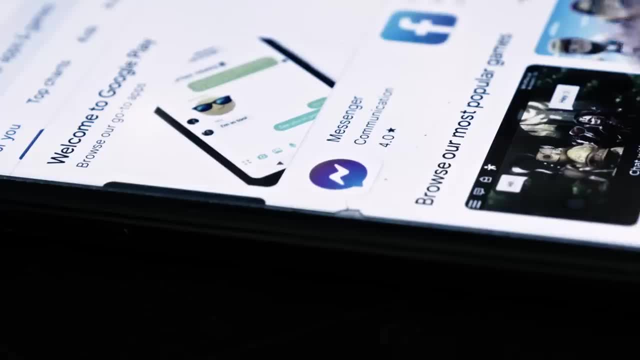 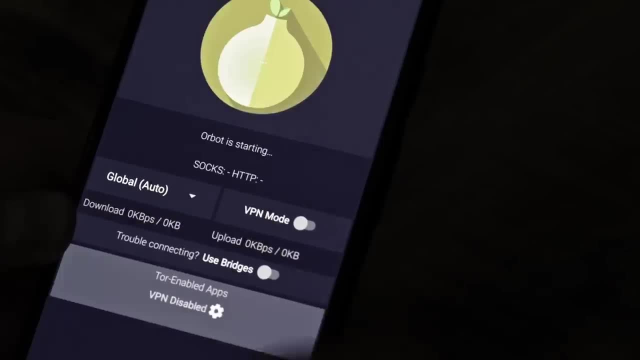 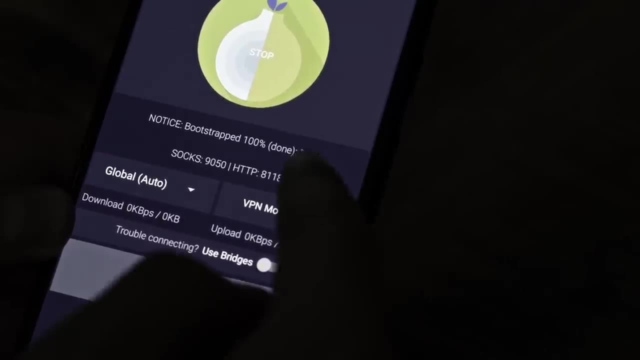 is no accountability, even in case of malevolence. The problem with mobile apps is that you have to do a lot more to anonymize your account creation. By the very least, you should route your app traffic through Tor. This can be done with Orbot. When you install Orbot, launch it and select VPN. 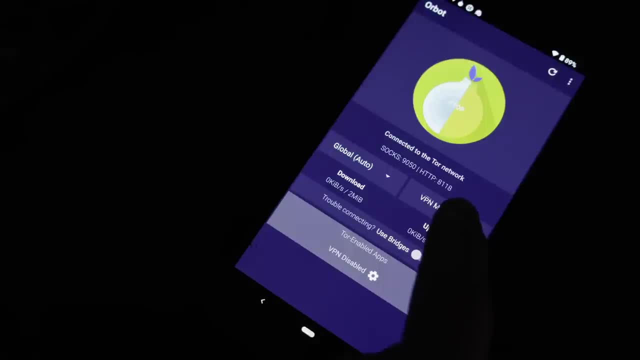 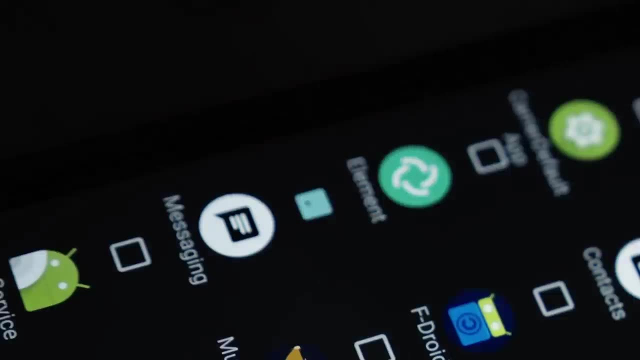 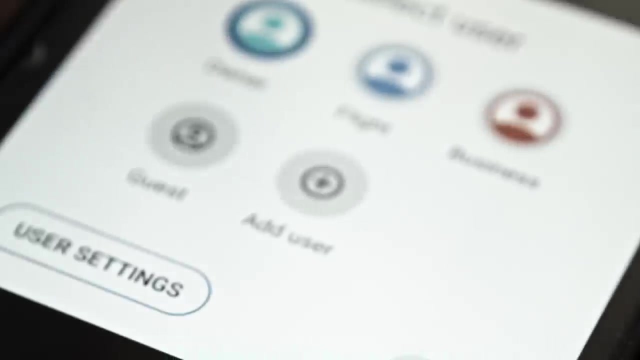 mode and choose your Tutanota and ProtonMail apps. This will route their traffic through the anonymous network and hide your location. You should torify the traffic for all of your anonymous accounts you will later intend to create. If your intention is to create an anonymous account, that can't be. 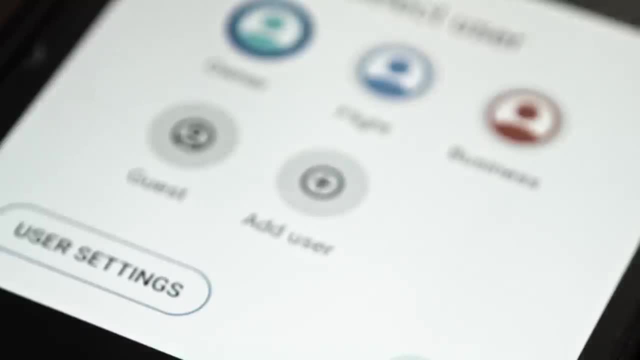 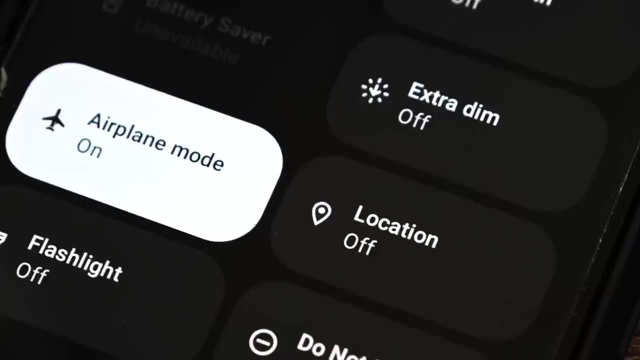 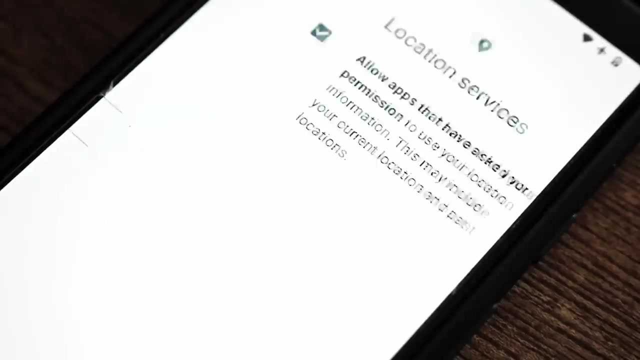 linked to your personal activities. you should create a separate user profile where you install these apps from scratch. I recommend doing this on GrapheneOS because this setup is the most secure and private and user profiles are more isolated on GrapheneOS than anywhere else. 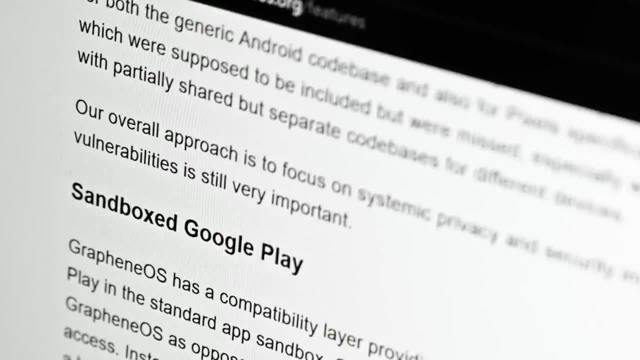 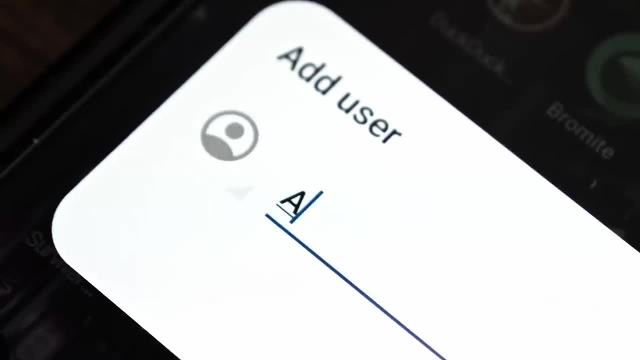 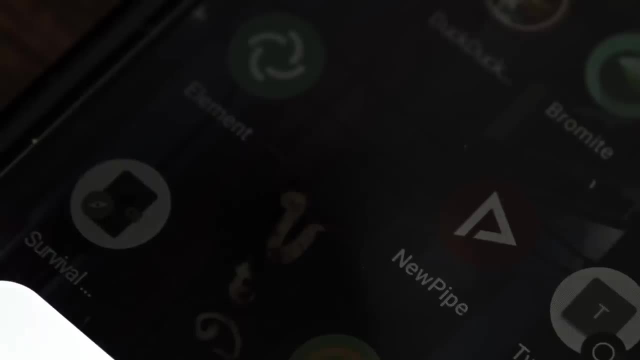 Your phone will also be completely de-googled, giving you total control over what apps have access to what types of your data. The second best option is to create a separate user profile on a stock Android phone, but this isolation isn't going to be as strong as on GrapheneOS. 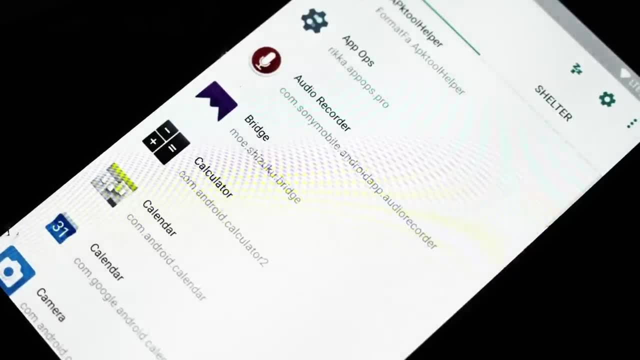 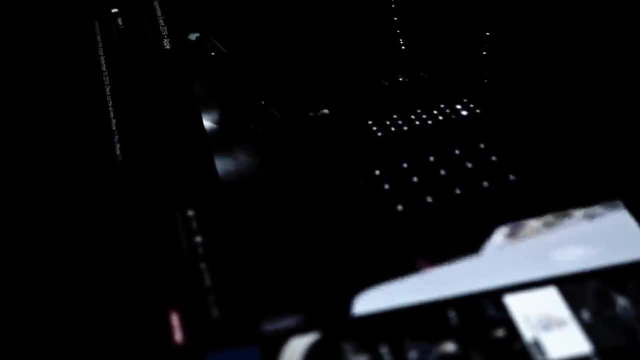 The third best option is through work profiles, which can be done with an app like Shelter, but that's again on Android. iPhones don't offer profile separation features and it is virtually impossible to verifiably isolate profiles on iOS with any tool I recommend. 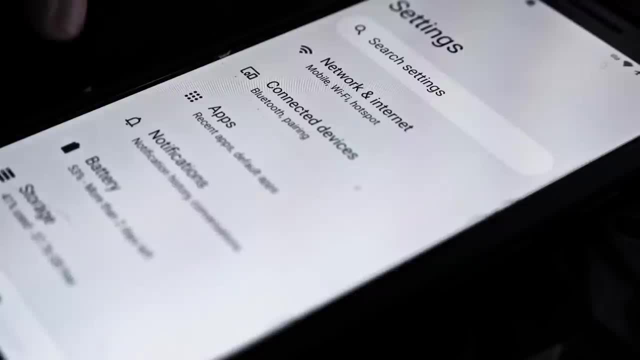 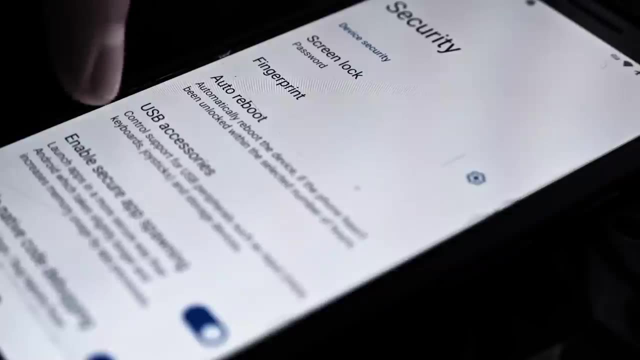 getting a new device or switching to GrapheneOS. A mobile setup is actually recommended if you also need to maintain high security and could have your anonymous identities targeted. It is important that you download these apps as anonymously as possible. Strong anonymity can only be achieved. 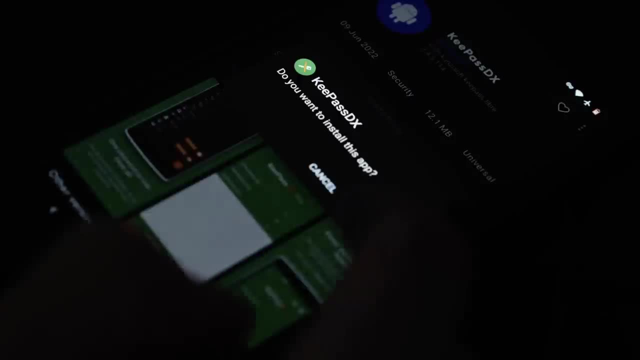 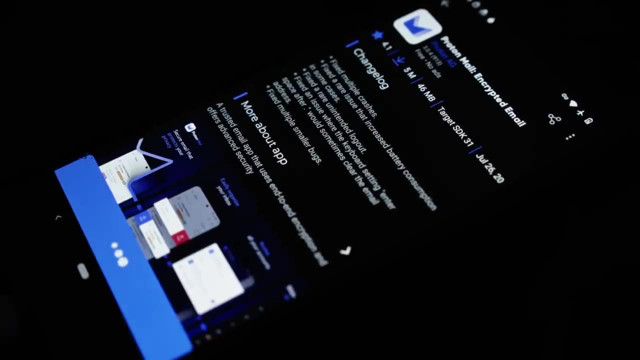 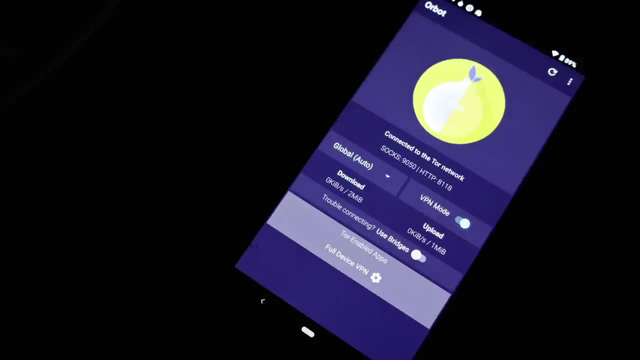 on Android by downloading apps from the Aurora store or FDroid instead of the original Google Play Store app. Aurora will let Android apps without a Google account and if you do this in a separate user profile over Tor or a VPN connection, it can actually be completely anonymous. 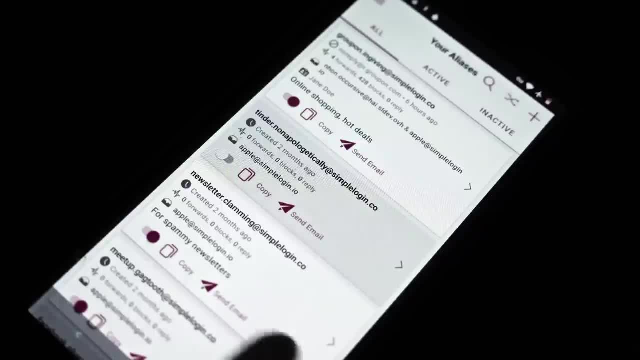 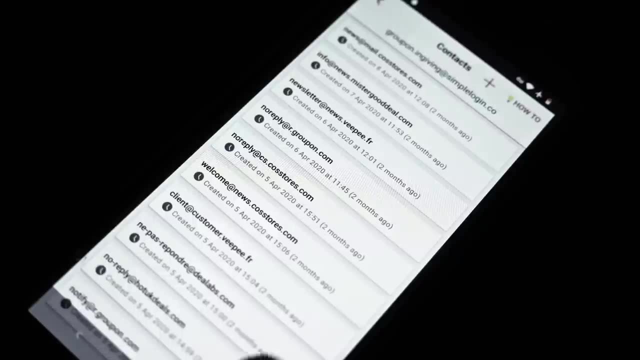 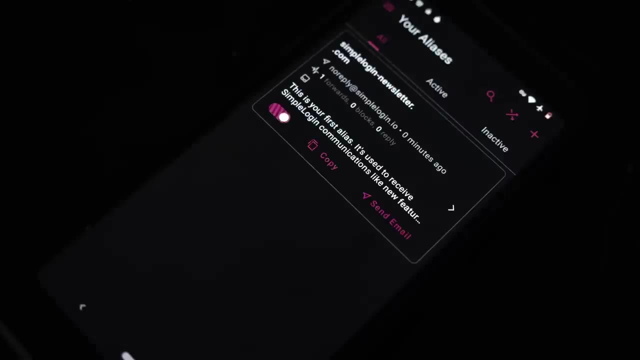 Now that we have anonymous email accounts, we can take this to another level by creating one-time email aliases. There is a range of options to choose from, both paid and free ones. With your anonymous Tutanota and or Protonmail accounts, you can sign up for a free email alias service. You have two options again: add an. 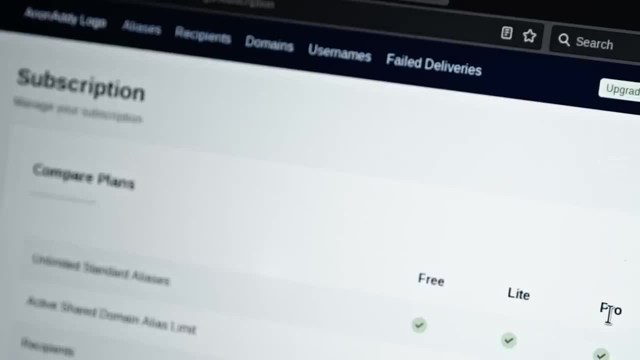 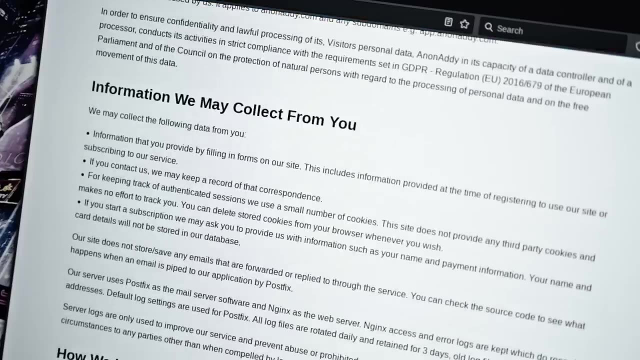 addy or simple logging. They're both similar in their offering of free and premium accounts. Here is an important note about email aliases: Service providers will have access to your email metadata and message content. That means they will be able to correlate what you use each email alias for, If there is any. 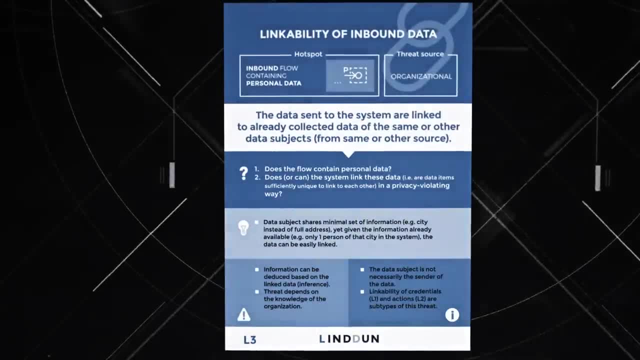 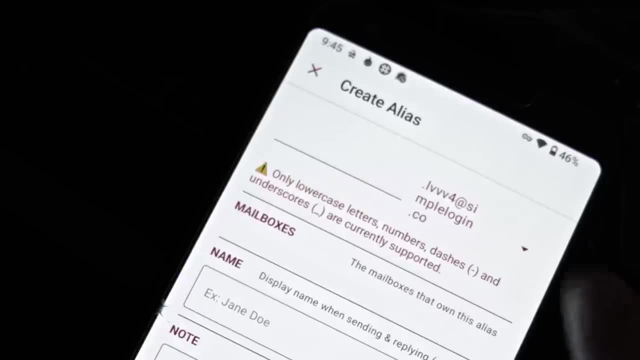 personal data flowing through these email aliases. the providers will be able to see it. The point of email aliases is not to use them for confidentiality, but rather as throwaway addresses you can give to services you don't care about in the long term. If you want to go for a paid option, it might be most. 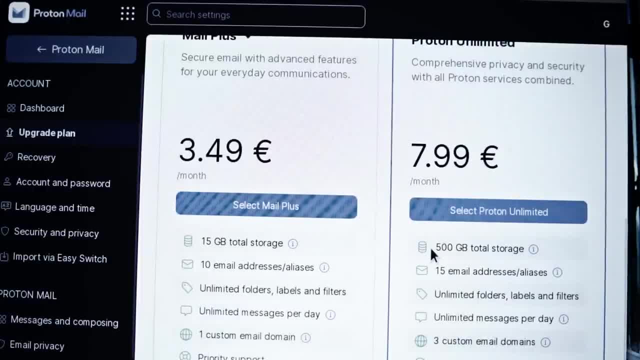 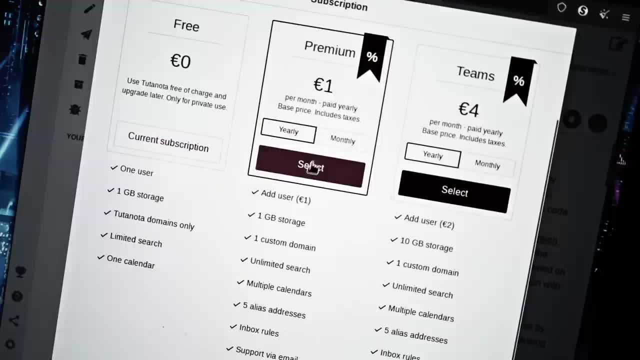 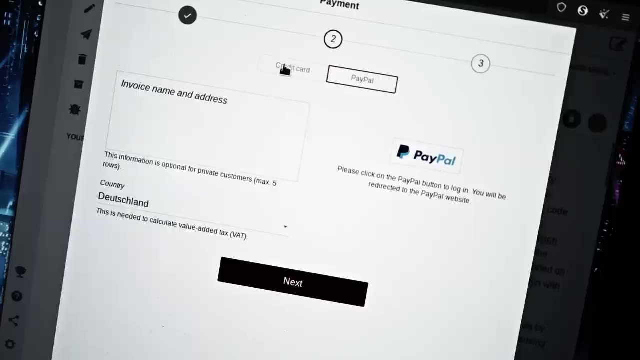 useful to purchase email aliases directly from Tutanota and Protonmail. You will have to subscribe to a paid plan for a monthly fee to get more aliases. If you are going to do this, don't provide any personal billing details. so this means no PayPal, debit card or bank transfers. They are completely out of the 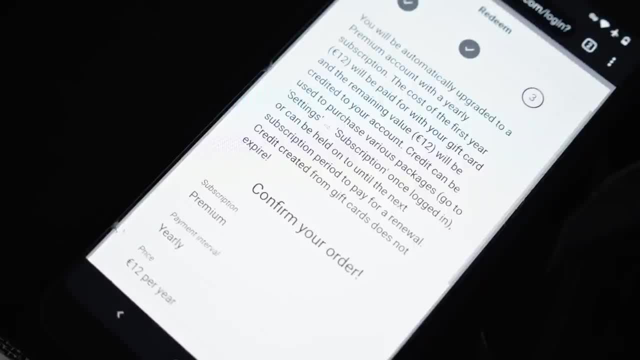 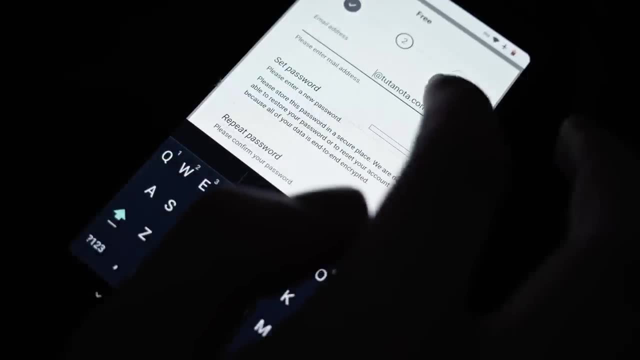 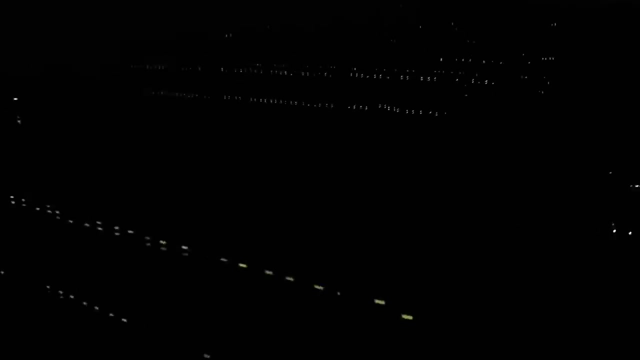 question here. Protonmail accepts cash and Tutanota accepts Nero, an anonymous cryptocurrency. I recommend Tutanota with Monero, as this is the fastest way to upgrade your anonymous account. I don't recommend Bitcoin for anonymous payments, as Bitcoin is actually publicly traceable and companies are paid money for chain. 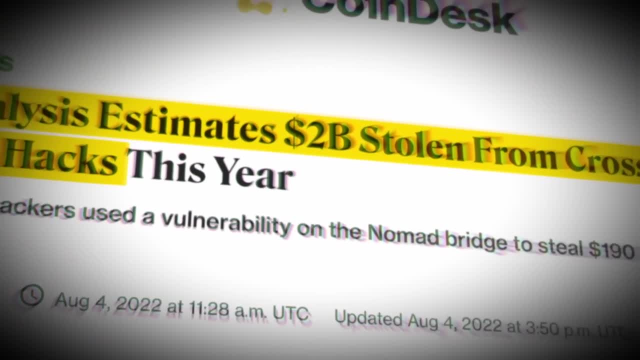 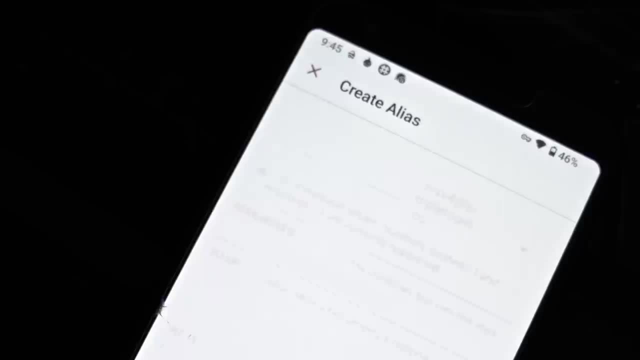 analysis. Chain analysis means they can track down movements of every single Bitcoin transaction. It is more private to send cash or use Monero. You can generate a new email alias for every specific use case. All the emails you receive will be in one unified form. 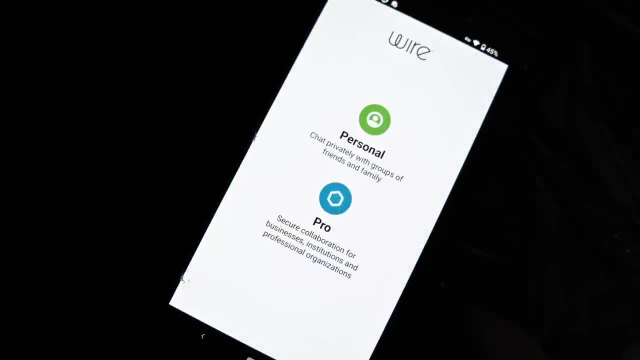 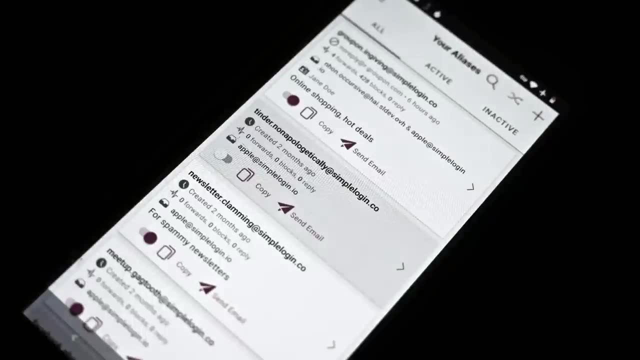 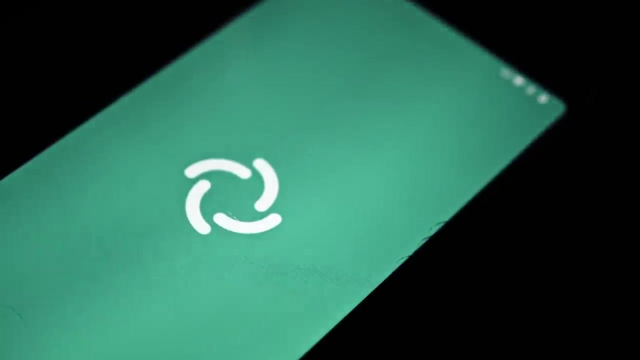 This setup is useful if you want to compartmentalize your online accounts that you intend to run for the long term. What you can do with an email alias service is to have a unique alias for each new anonymous account you create for other services. There is a number of services worth trying to create an. 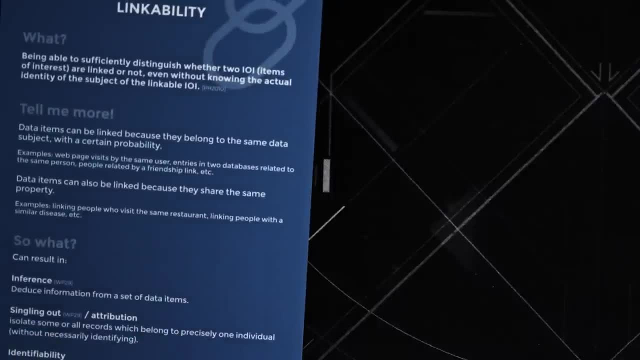 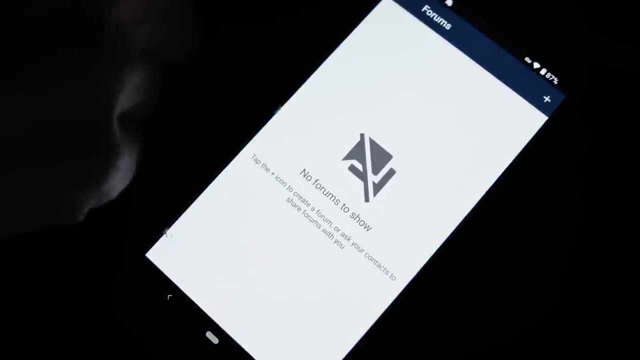 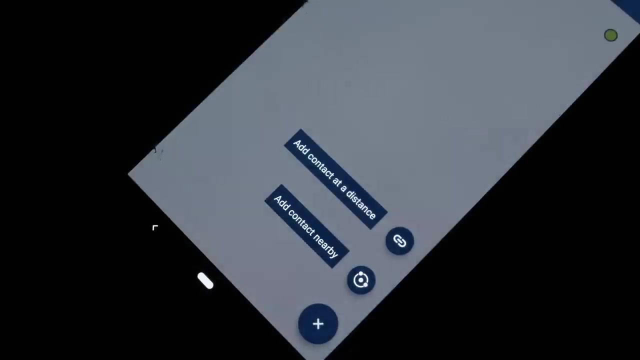 anonymous account for Some services will meet all of the prerequisites to mitigate all linkability and identifiability threats. Completely anonymous accounts for real-time communication are briar and onion share. It is unlikely your contacts will already use any of these, so you will need to find a secure way to communicate your new details with them. 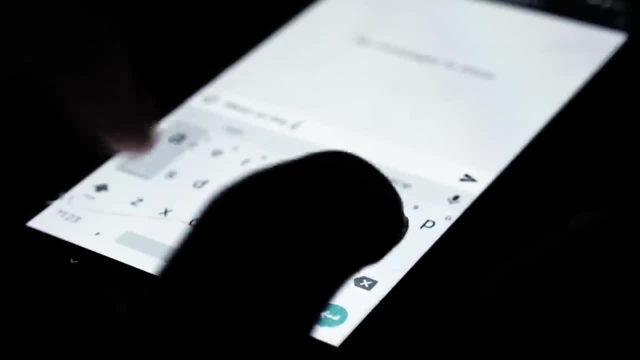 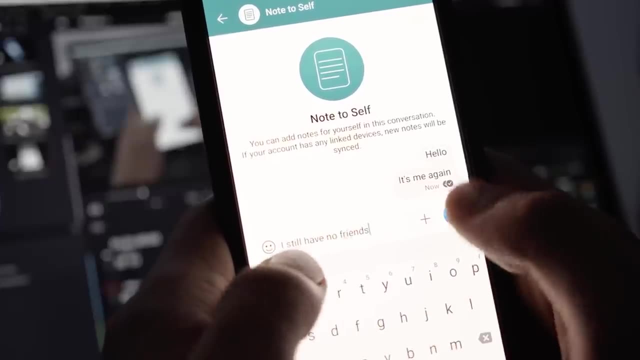 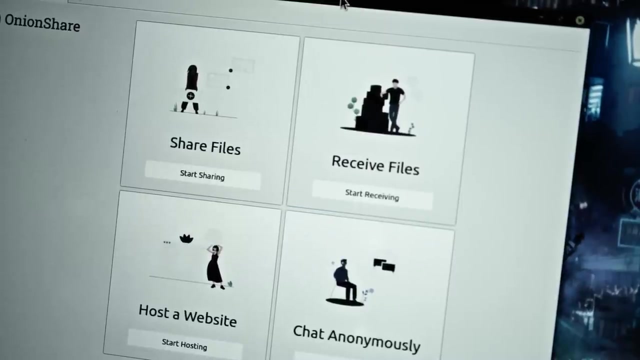 For briar. you can send your address to your contacts in an encrypted message with your anonymous encrypted email address. If you and your contacts both have signal, then you can send your briar address in a disappearing signal message too. Onion share is interesting because it allows you to create ephemeral chat. 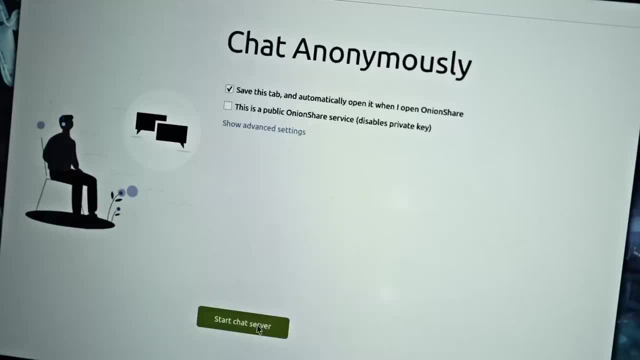 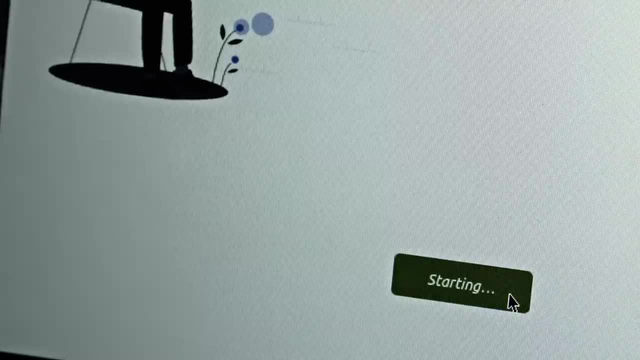 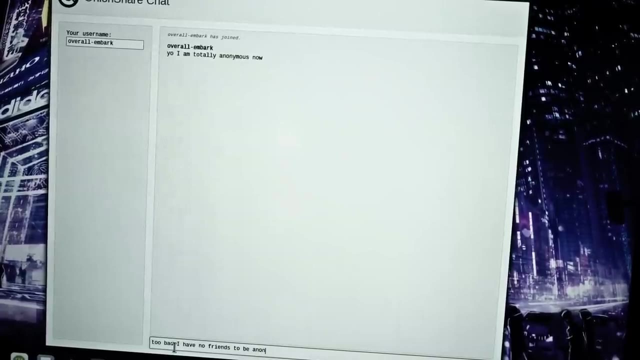 rooms. It will be hosted anonymously on the Tor network and will complete the list of accounts for people who use it. Some chats will simply disappear once you close them. All you need to do is start a chat server and share your public address and a private key with your contacts. Your contact only need to open. 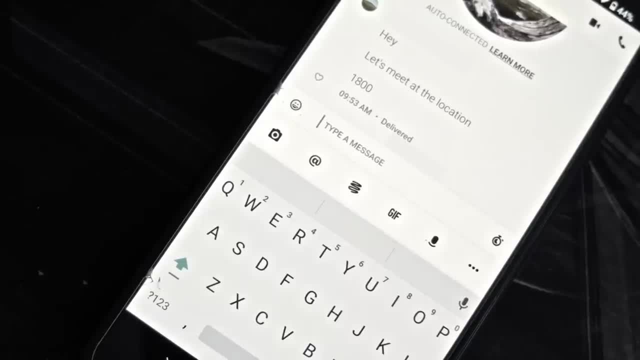 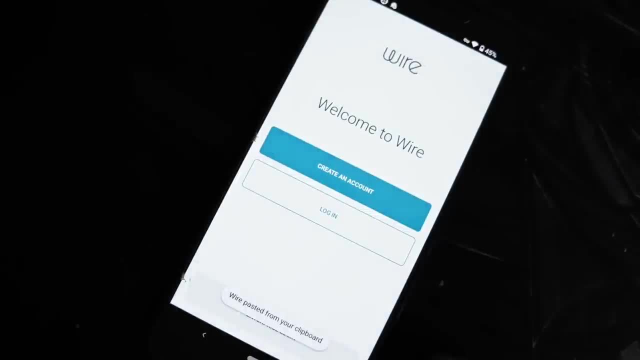 this link and enter the private key from the Tor browser. No accounts are needed for onion chat. Wire is another messenger that can be downloaded and used anonymously. It is available on FDroid, which means no Google Play is required, and it allows email aliases as well as. 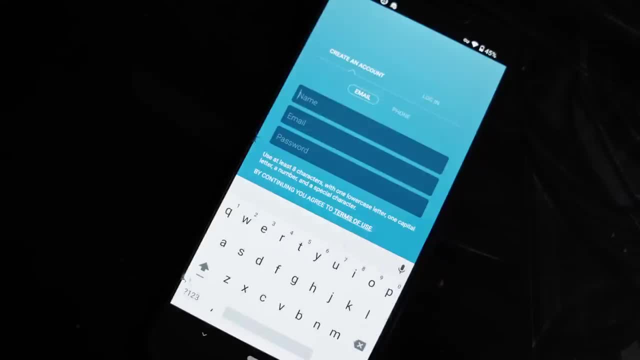 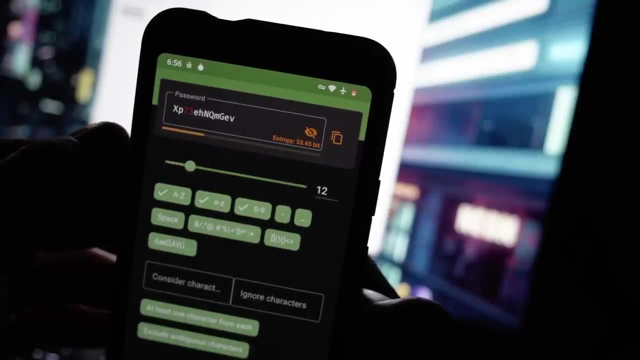 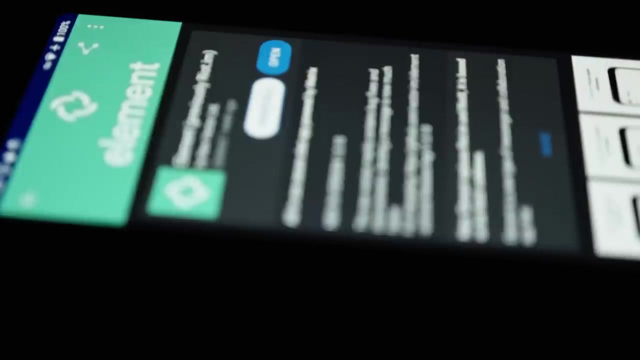 corporate clients. but if you intend to use it individually, then it is highly recommended to use it completely anonymously, always over the Tor network, with a randomly generated username-password combination in the password manager and with anonymous email. alias Matrix is another great service that can be used for messaging: voice calls, group chats. 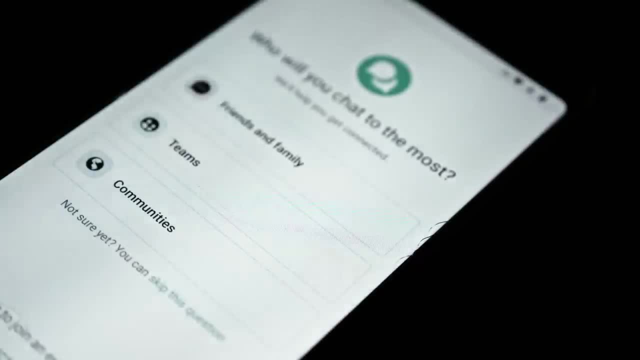 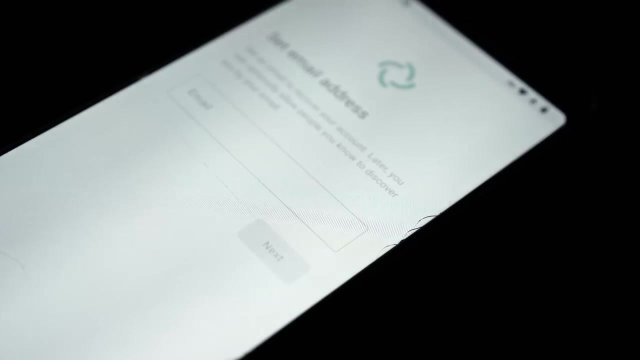 or chat rooms. There is a popular Matrix client called Element that can be fetched from any popular app store, including FDroid, which means it can be installed anonymously. The whole account creation and usage process work with no issues over Tor. This makes Element a very solid choice for anonymous, encrypted communication. 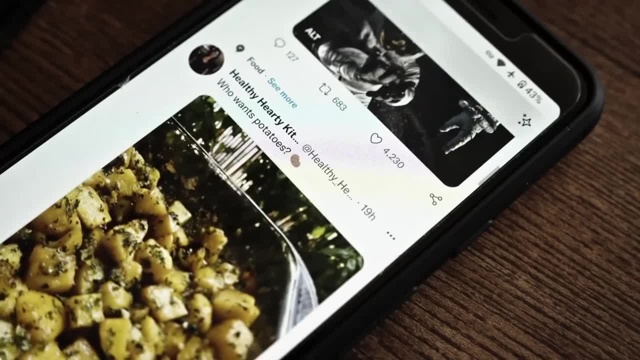 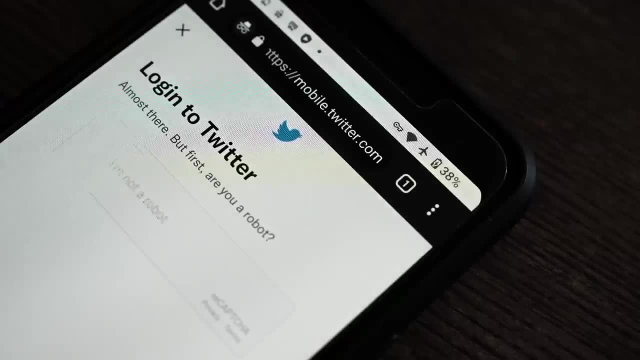 When it comes to social media accounts, using Tor or a VPN for account creation might get your accounts flagged and suspended before you even get to use them. You might try your luck and score occasionally, but in many cases you just won't be let.